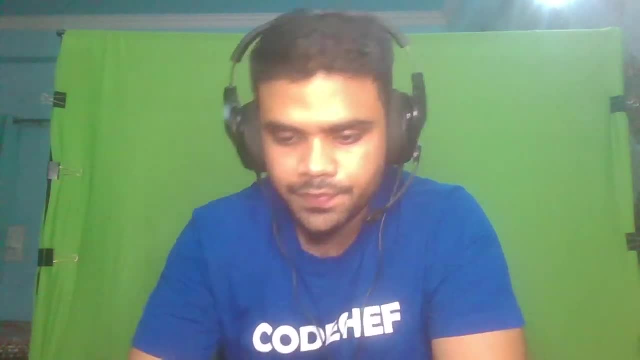 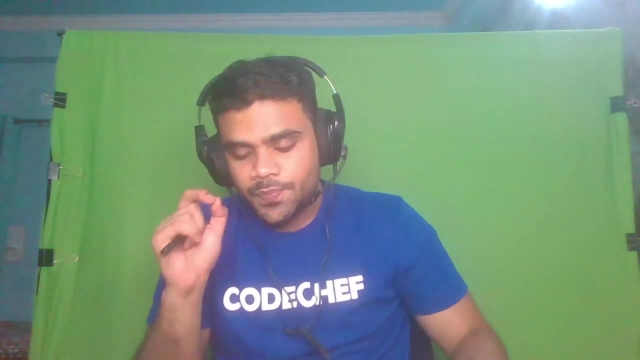 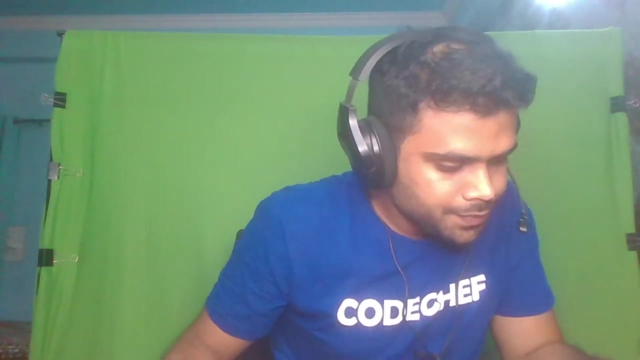 least kal wale log thod bau. join kar jayen, Then we will start. Okay, This is the lecture 2.. Yesterday we covered the lecture 1.. In the lecture 1, we saw what greedy strategy is, what greedy technique is and how to approach problems using greedy strategy. Hi Siddhi. 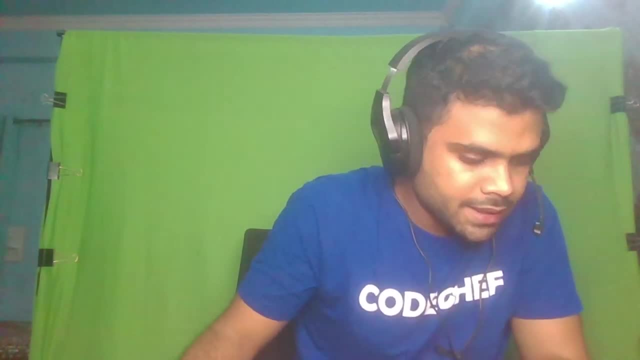 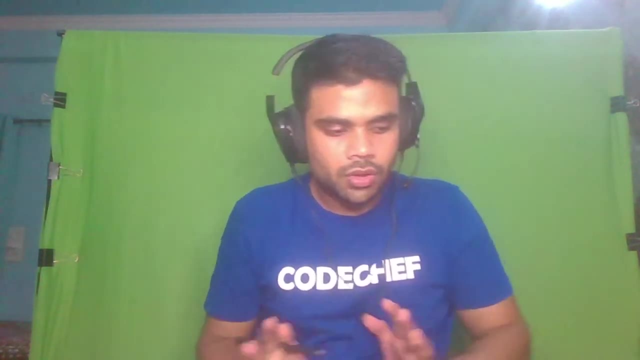 Bhanushali, Hi Shivansh Gupta, I was there yesterday Amazing, So I hope aapne questions kar liye hongi kal wale, Jo bhi humne class mein kar waye the You were able to solve. 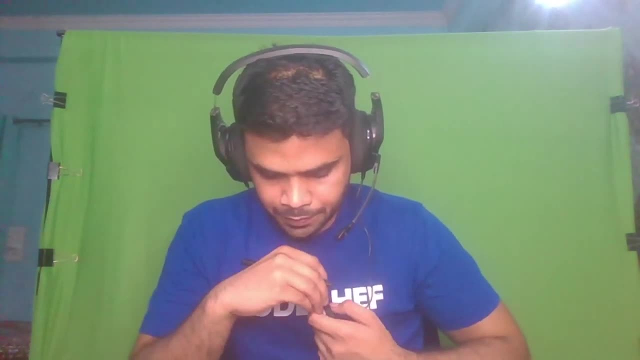 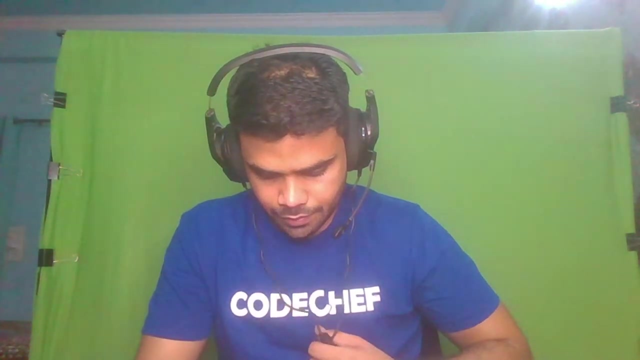 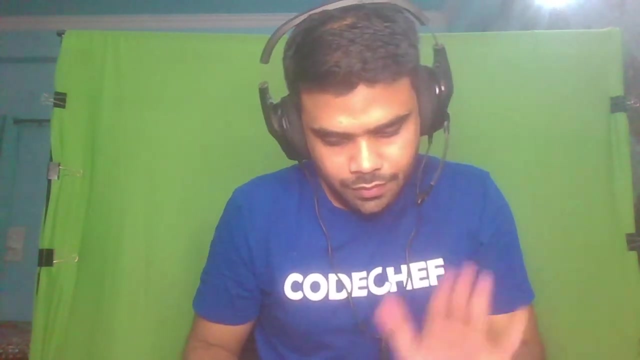 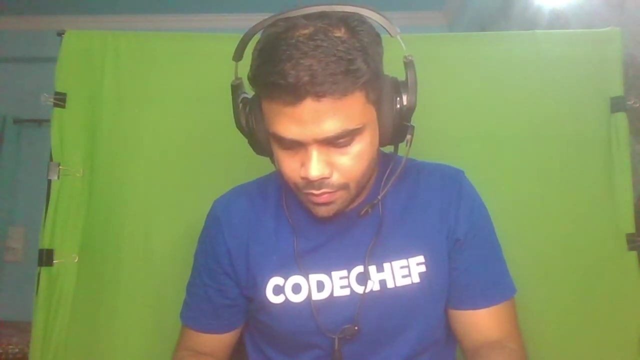 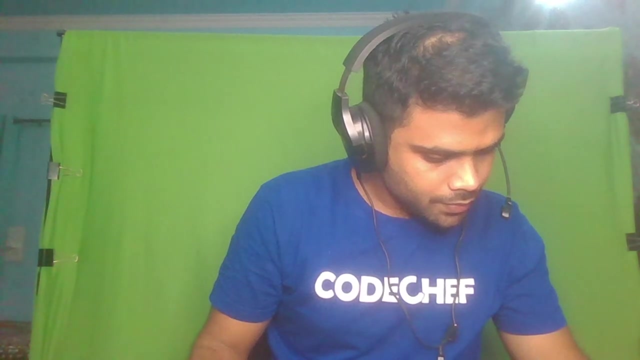 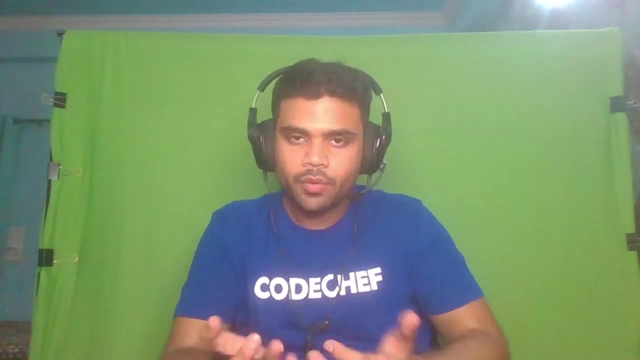 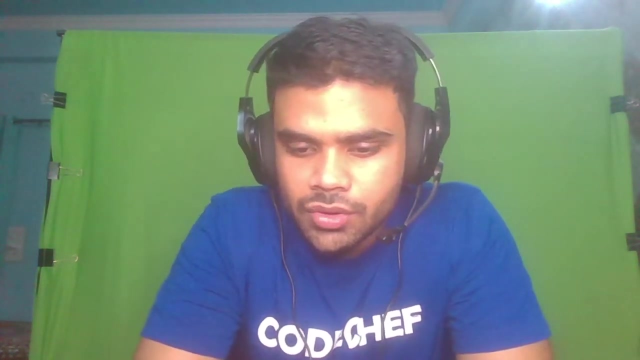 all of them right Submitted as well. Awesome, Nice, Yeah. Meanwhile, let us let me just cover a few important points that we covered today. Kal hum logon ne dekha that mostly whenever we are solving greedy. so either we sort the 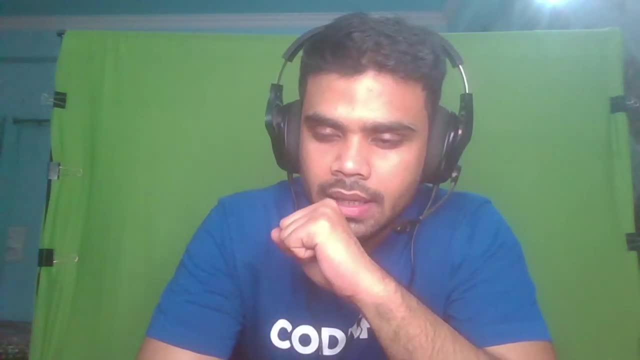 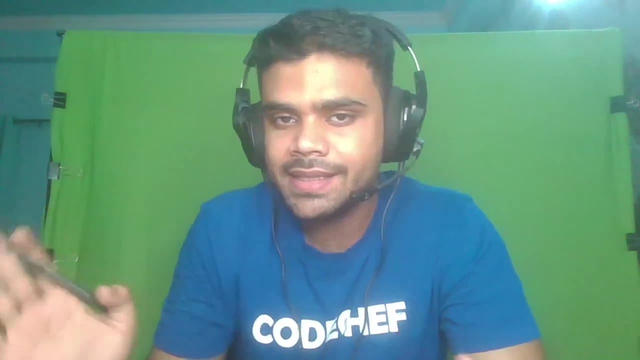 given input Hum usko sort karte hain. Okay, Ya, fir hum usme kuch search kar rahe. hota hai, either the maximum or the minimum. Okay, Sorting both ways. Ascending order: me bhi kisi kisi. 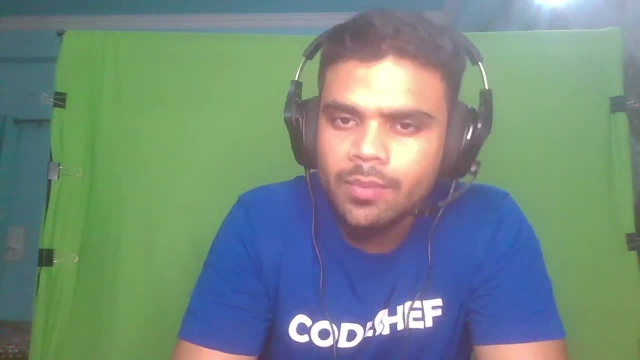 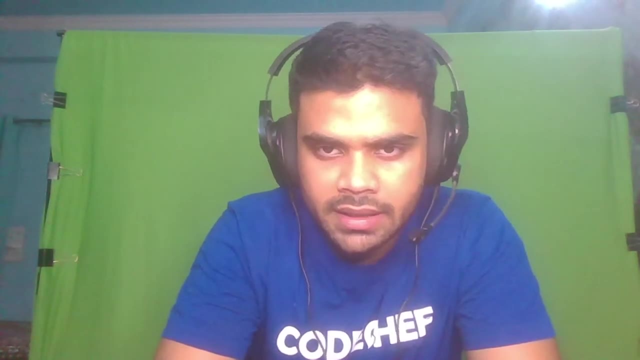 situation me sort karna padta hai, Descending me bhi sort karna padta hai, Aur kahi baar hum log priority queue use kar rahe hota hai. Sometimes we are using priority queues as well. Okay, Yeh generalize maine aapko bata diya. This is not. 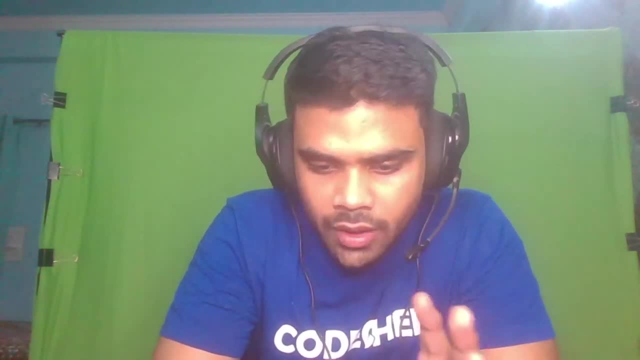 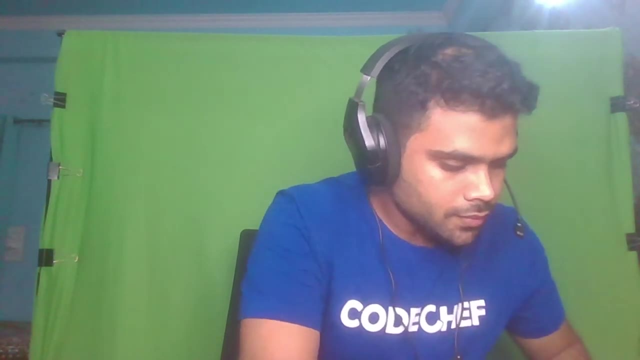 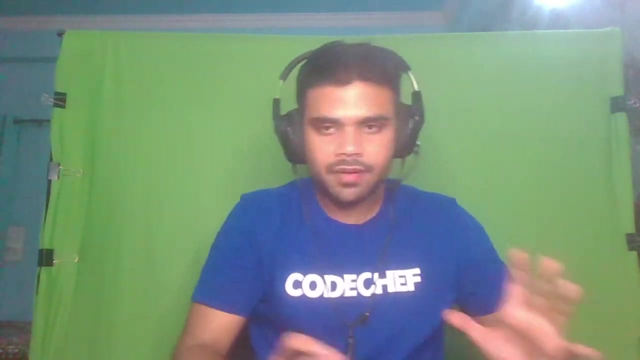 Koi hard fast uska rule nahi hai, ki hamisha yeh he hota hai, But this is the generalization, jo ki zyadatr use hoti hai. Okay, Chalo, I guess now we can start. Okay, Everyone do. 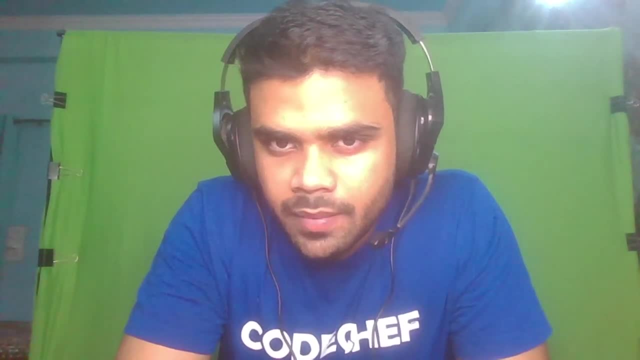 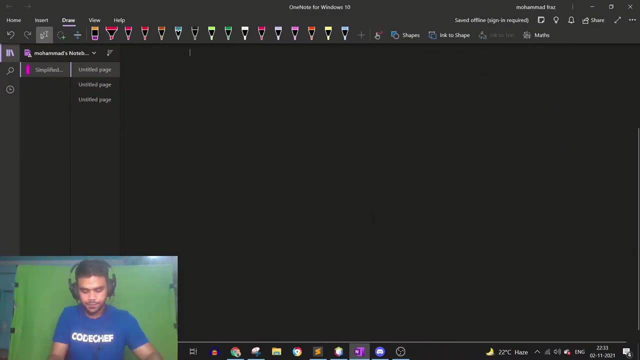 like this stream as well. Let me minimize this. Yes, I think it is fine. Okay, So as So. I am Faraz, and this is the lecture number 2 of our Greedy series. In this series, we are learning that how to use greedy technique to solve multiple questions. 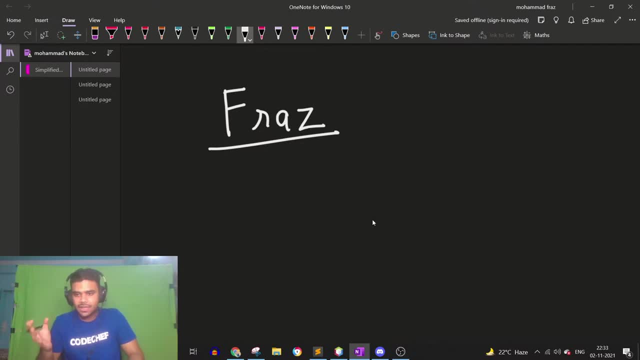 So today we are going to do the activity selection problem with intuition. So this is, we are going to cover the activity selection problem. but this is not just a problem. There are multiple variations of the same problem as well. There are many variations of the same problem, and once you learn how to intuitively think, 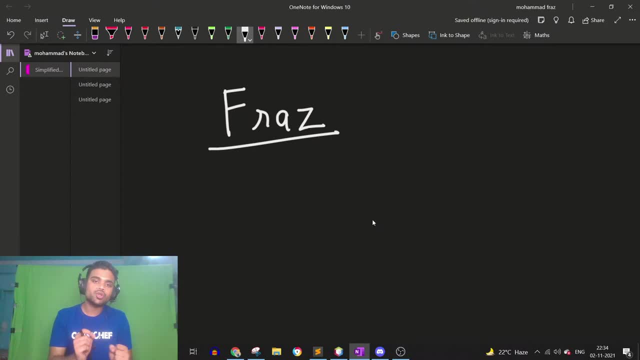 how to develop the algorithm to solve this problem. you will be able to solve other problems as well, And this is the plan, this is the agenda: that you should understand the intuitions rather than the questions. it is better to understand the intuitions and then solve the problem. 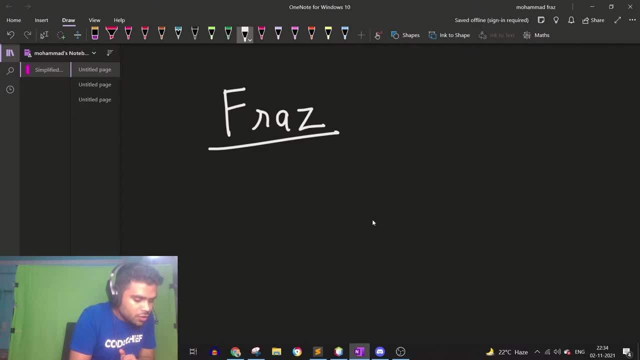 There are many more questions based on that, So let me give you the question: what the question is. So the question is that there are multiple activities, okay, multiple activities that you can perform, alright, And each activity is having a starting time and an ending time. 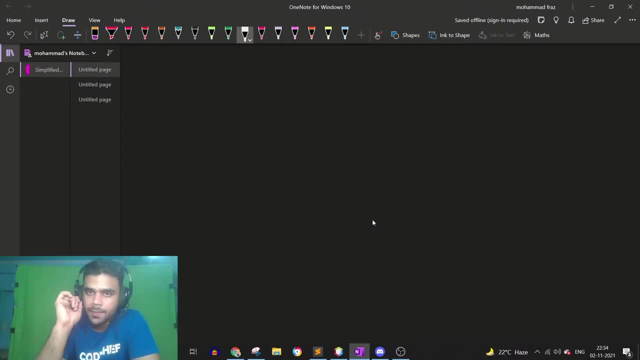 Activity ke shuru hone ka time apko pata hai. activity ke khatam hone ka time apko pata hai theek hai. There are multiple activities given apko, So you have to select multiple activities that you can do. okay. 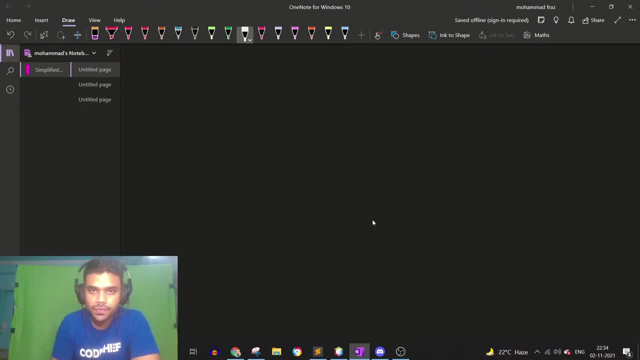 So out of the given activities you have to select the activities that you can do. Acha abhi yaha par problem kab aati hai? The problem is, you cannot select two activities which are overlapping. For example, sabi log dhyahansi questions sulle na, because I am not writing it down. 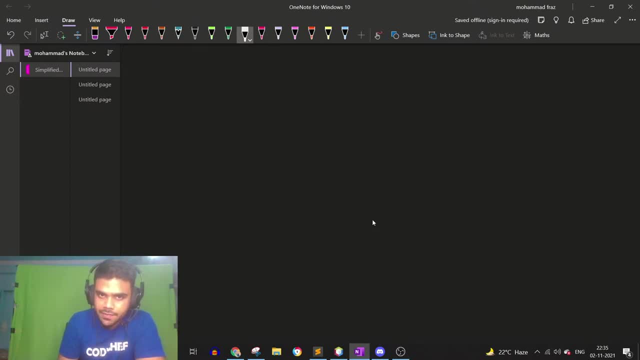 So the problem arises when there are overlapping activities. Okay, Ek particular activity hai. okay, This is starting at, let's say, one: One se lekar ye activity apki three tak chalti hai. Ek activity apki two se start hoti hai, starting from two. 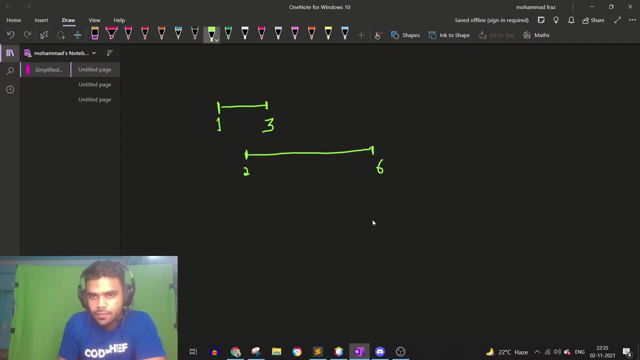 Aur ye apki six tak chalti hai. Okay, Phir ek aur activity apki let's say four se start hoti hai. Ek activity apki two se start hoti hai, Starting from two, Aur ye apki six tak chalti hai. 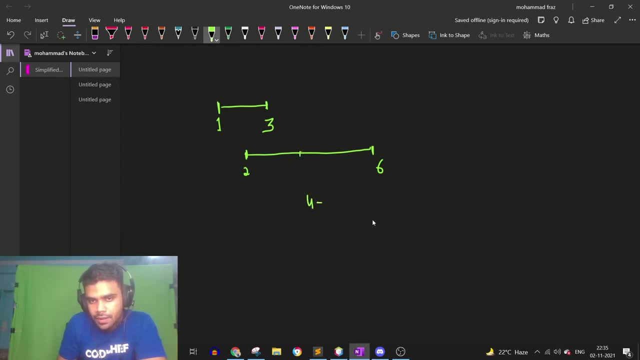 Starting from two third Okay, Aur ye apki da baat hoti hai, Okay, And wo five tak chalti hai. So in this case, if you select the activity, this is the activity number one. this is the. 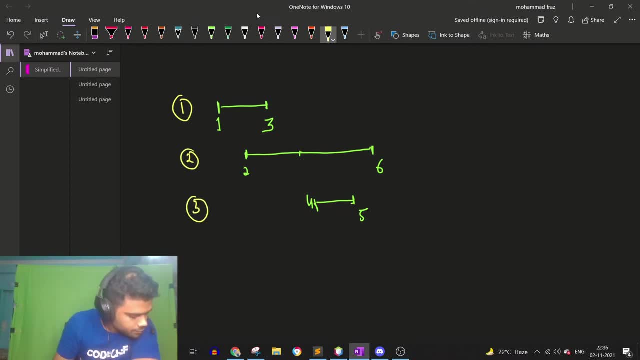 activity number two. this is the activity number three. There is no prerequisite. There is no prerequisite at all. Just watch it with focus. Focus is the only prerequisite here. okay, So there are these three activities. Okay, activities you have to select. you have to select as many activities as possible. 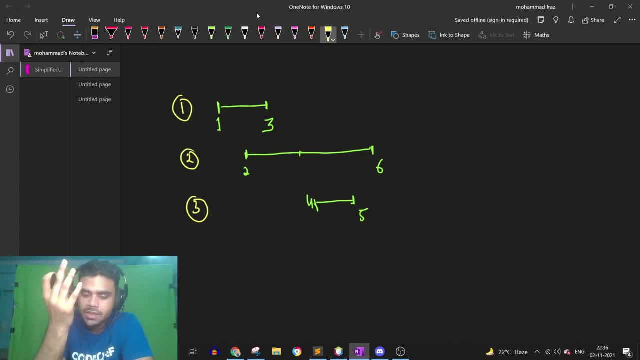 you cannot select activities which are overlapping because you are doing one work, let us say, this is watching movie, this is, let's say, this work can be done for 4 hours: 2 hours for movie and 4 hours for study. this is study and this is playing football. 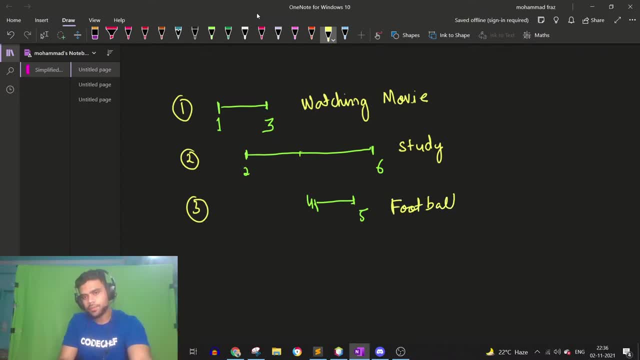 okay, out of the three activities you can select- you can select as many, not as many. you can select only the activities which are non overlapping one activity. if you are doing, let us say 1,2,3, if you are watching movie, you cannot study. so it is not that you will finish watching movie on 3, then you will start studying from. 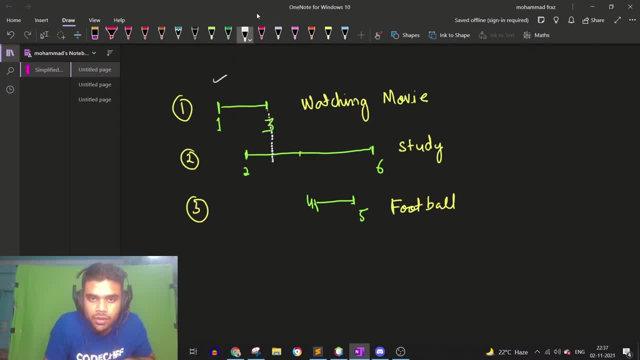 3. no, you are not allowed to do so. you will not be able to select this particular activity because you have to do activity from start to end. okay, if you have done one activity, then you have to do activity from start to end. i hope question is clear now. 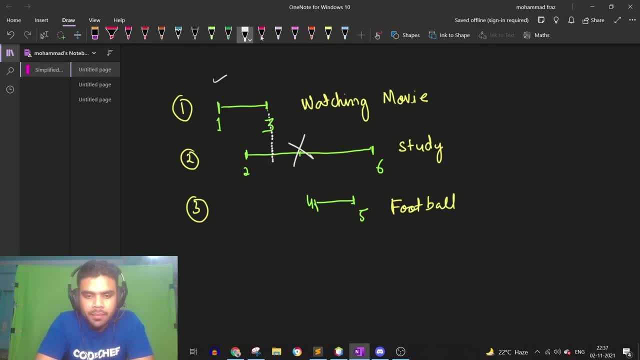 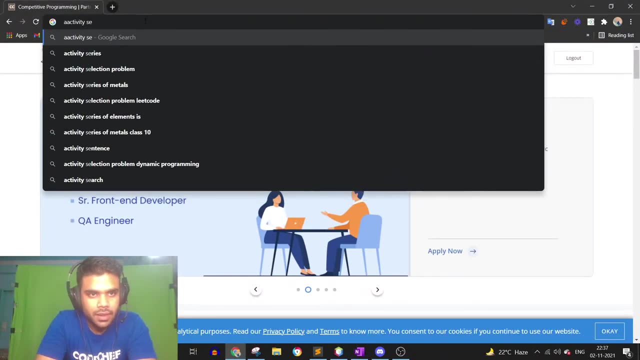 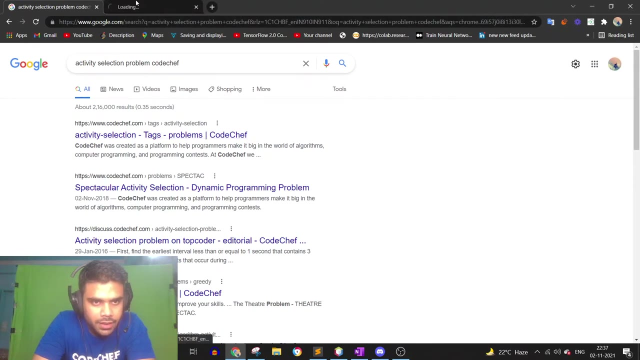 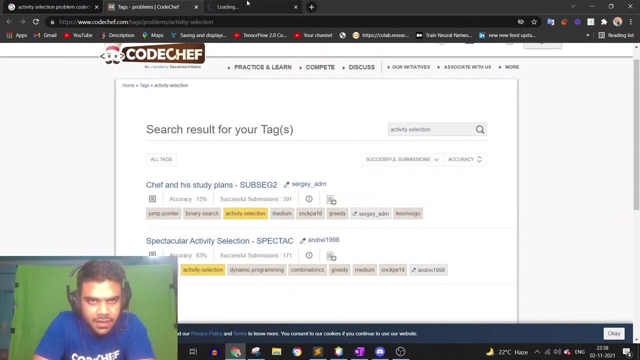 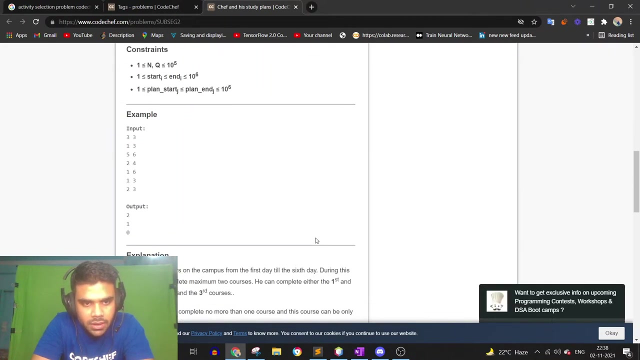 problem link: problem link. let me search here. activity selection code: chef- activity selection problem code: chef. activity selection chef and his study plan. let me see if this is the same problem or not. but meanwhile let me just explain this one. okay, this same problem, i guess. wait a second. 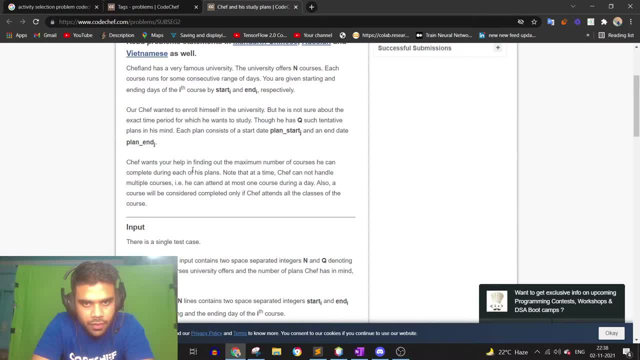 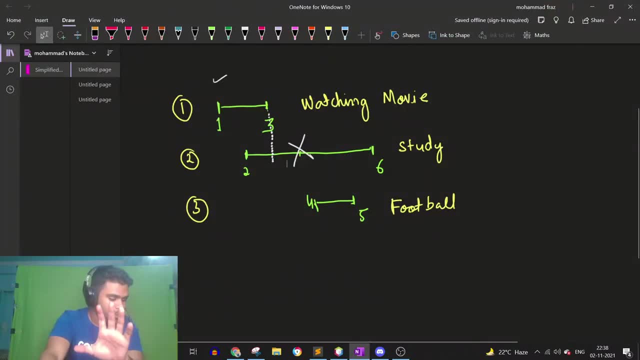 wait a second maximum number of the courses he can complete. okay, okay, nice. i think this is the problem. this is the problem, but let me explain it over here. let me explain it properly first, and then we will move ahead. let's go so here. activities are given their starting time and ending time is given. 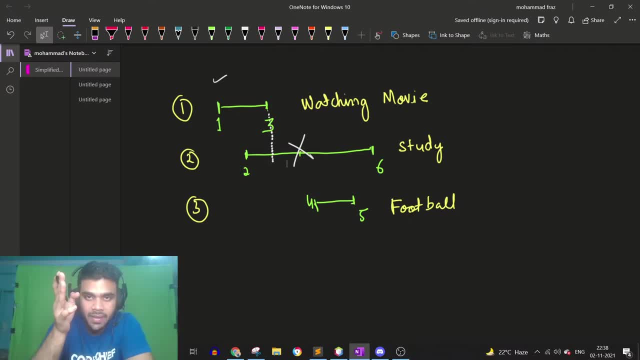 you have to tell me how many activities you can select. here it says how many activities you can select at maximum. if you want to maximize the number of activities that you can select, which activities are you going to pick? tell me you are going to select the activity number two. 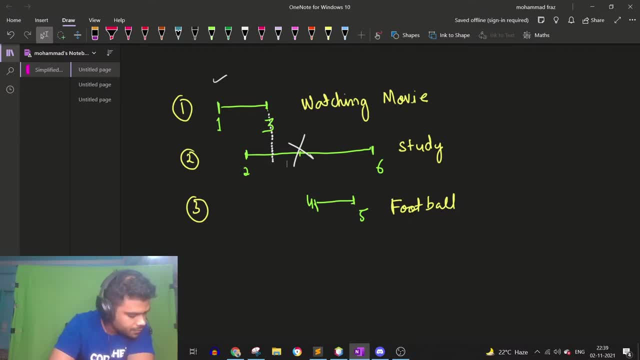 dev brad dev brad. mishra, are you going to select the activity number two? and abhay rathee, are you going to select the activity number two? okay, abhay, you are correct. shubham, you are correct. chandan, you are correct, you don't have to study, because study. 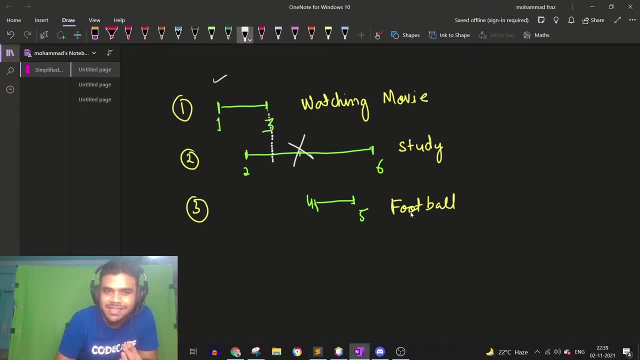 if you study, you are going to miss watching movie, you are going to miss playing football. so you don't have to study, you can watch movie first and then play football. this is the correct answer. answer is two number of activities you can select and which activity is activity number one and activity number three? you can select. 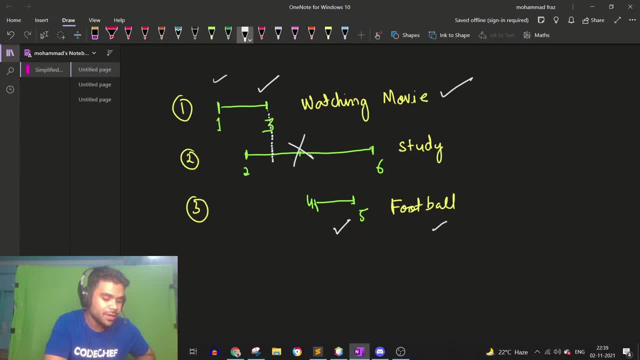 so how did you go for it? how did you think about it? can you just tell me what is the intuition? what did you think about it? tell me many people you will answer wrong. so that's why you have to think about your answer a little bit, think a little bit. 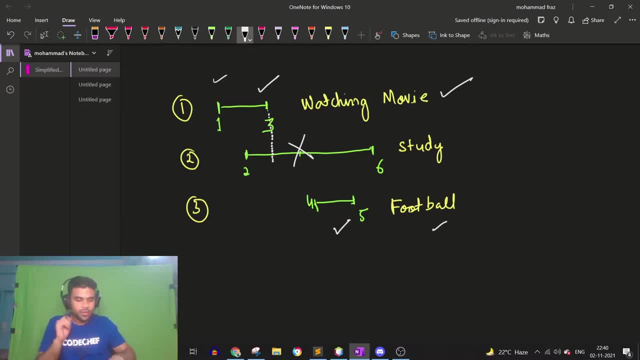 because many people answer wrong as soon as they ask this question. i have already given the warning, so just think and answer. on what basis have you selected the activities? hi myank, hi, everyone those who are here. they can ask me the question if they don't know. 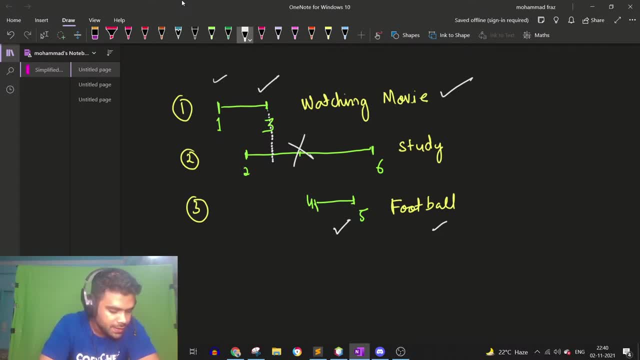 already what the question is: rohit chaubey, okay, okay, okay, i guess. okay, namaste, harsh namaste. no overlapping time between these two tasks. okay, dev brad mishra. no overlapping time between these tasks. that is fine, that is fine, but that is not the criteria to select. 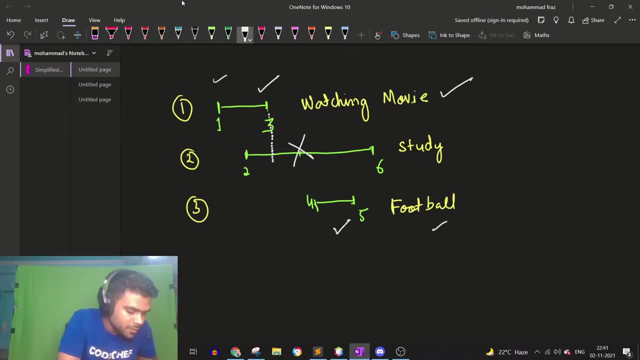 how will you be able to select based on that one and three are not overlapping, maybe on the basis of most number of non overlapping activities? see, no one gave the wrong answer. so how will i tell you now according to the finishing time of the activity? okay, okay, okay. 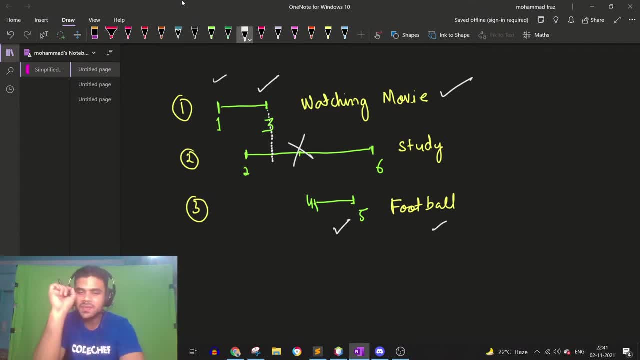 so you all know it okay. So lot of people say, start picking this smaller activity, start picking smaller activity. Is it the right logic? kya yeh sahi logic hai, ki choti activities ko aap log pick karo? kya lagta hai aapko? is it the right logic? if you agree with this, please write yes in. 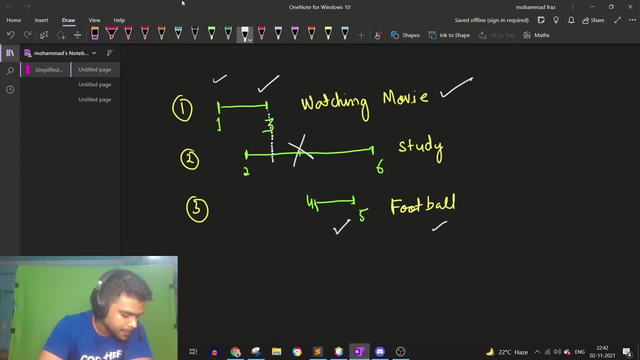 the chat Intuition ek baar develop ho gaye na ki greedy, kaise solve karne hai then? greedy is going to be very simple, the most simplest topic. dekho, tanuj ne bola yes and merum ne bola yes, but that is actually wrong. woh galat hai. why is it wrong? woh galat kyun hai uska. 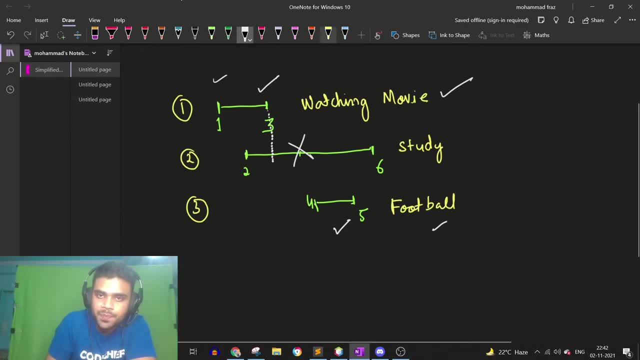 bhi aapko example deta hu. let me give you a quick example for that as well. ki woh cheez kyun galat hai theek hai, yaha par, dekho aap log. let us say, there is an activity which. 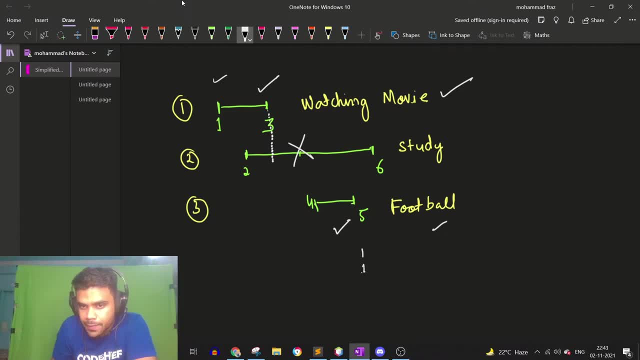 is starting at 1 and it is ending at 2.. Let us say it is ending at 6.. There is another activity which is starting at 5 and it is ending at, let us say, 7.. Then there is another activity which is starting at 6 and ending at 12.. 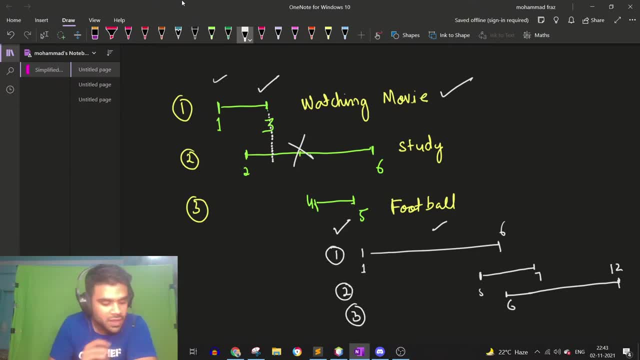 Activity number 1.. Activity number 2.. Activity number 3.. Activity number 4.. Activity number 5.. Activity number 6.. Activity number 7.. Activity number 8.. Activity number 9.. Activity number 10.. Activity number 11.. 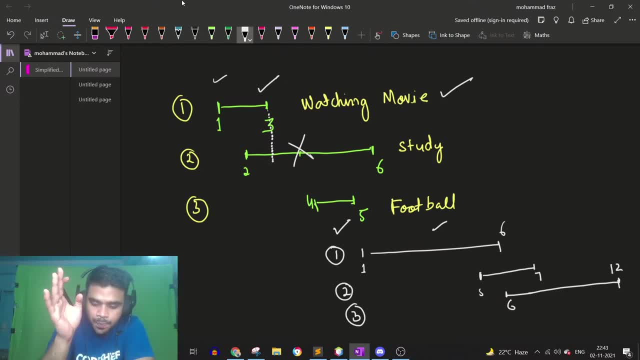 Activity number 12.. Activity number 13.. Activity number 14.. Activity number 15.. Activity number 16.. Activity number 17.. Activity number 18.. Activity number 19.. Activity number 20.. Activity number 21.. Activity number 22.. 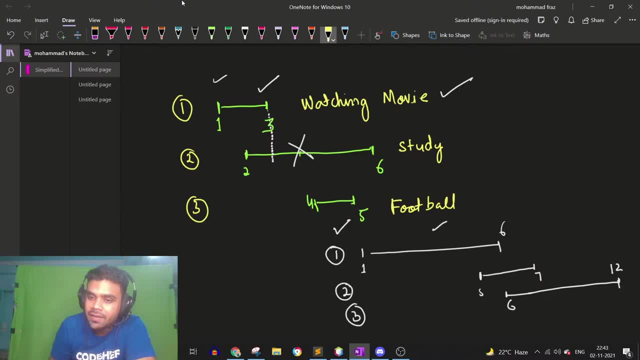 Activity number 23.. Activity number 24.. Activity number 25.. Activity number 26.. Activity number 27.. Activity number 28.. Activity number 29.. Activity number 30.. Activity number 31.. Activity number 31.. Activity number 32.. 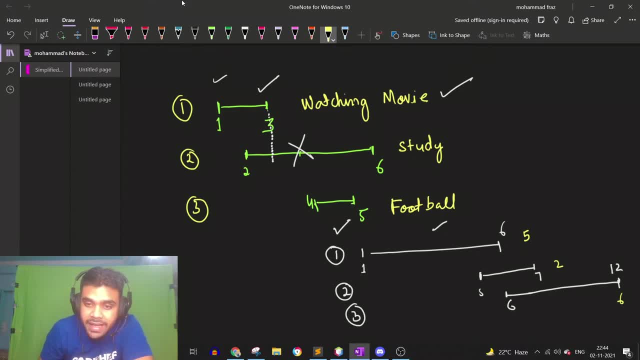 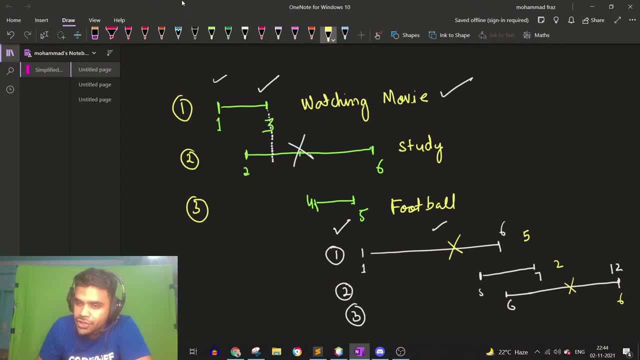 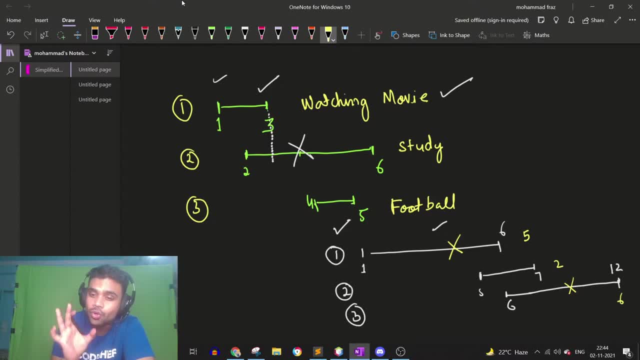 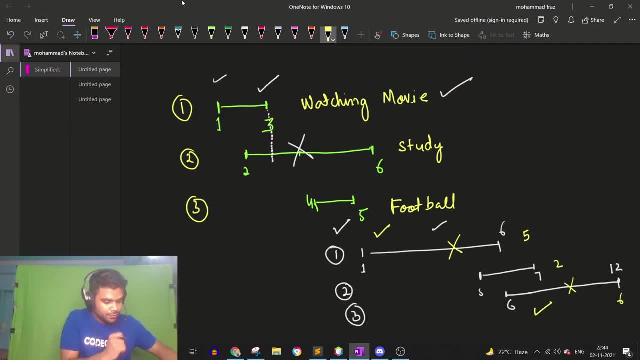 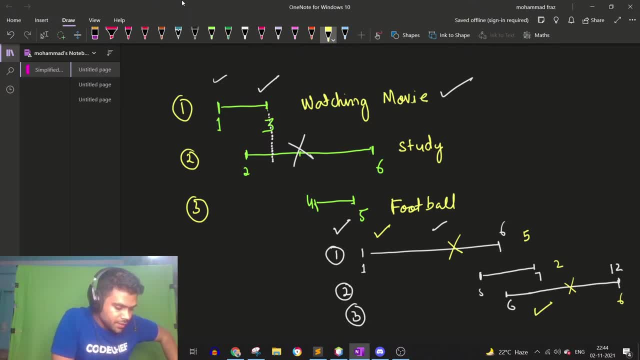 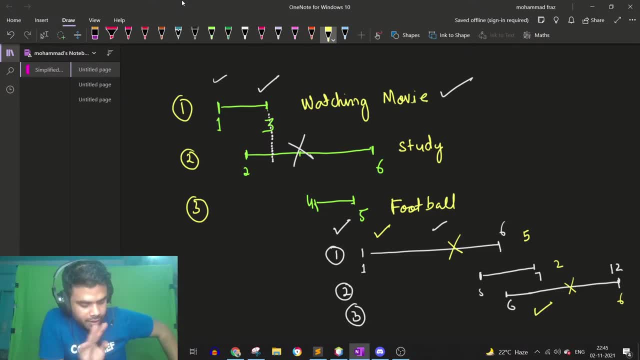 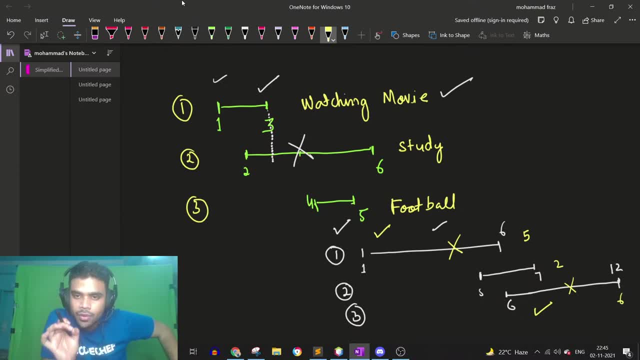 And we will be able to select the activities. listen carefully, with focus. We will be able to pick up activities only if we are free. If we are free, then only we will be able to select the activities. So we want to be free as soon as possible. 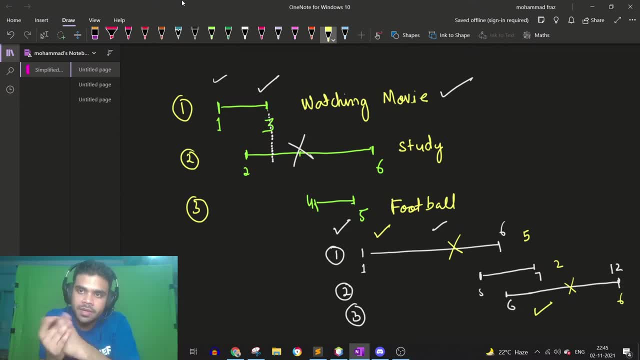 Let us say I am engaged right now And my engagement is till 11.30.. 11.30 is the class right. This is my engagement. Until I am not free, I will not be able to do any other task. 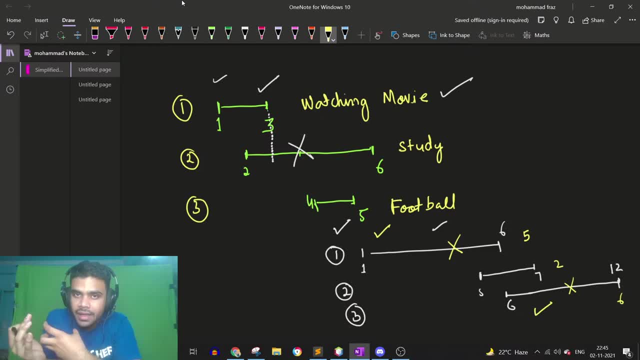 Got it. So this is the thing: I want to be free, So that I can pick up another task. To be free is the logic here. Brother, don't spam, Please don't spam in the chat. Okay, Danish, I will repeat. 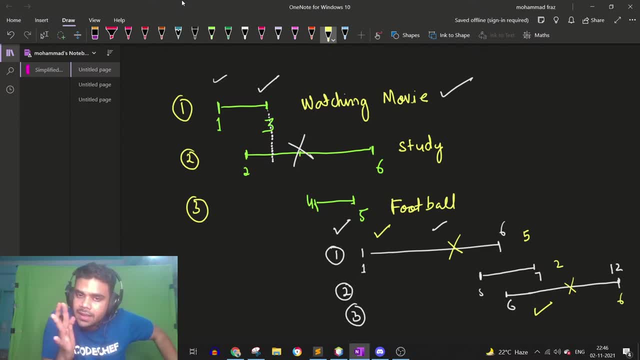 Don't worry, I will repeat the question. So, the activity that is ending first, the activity that will end first. I will be selecting that one. Okay, I will be selecting that one. Okay. Now there are two activities here. 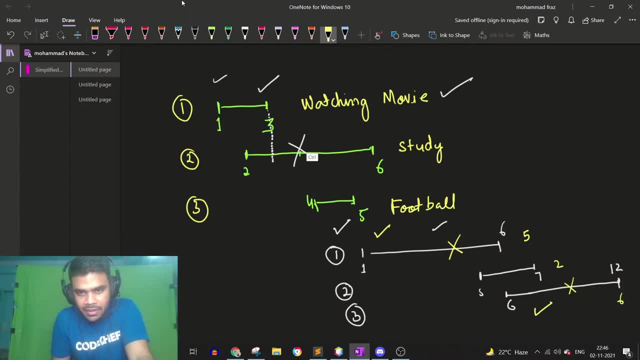 Let us say there are two activities. Now I will take a small example again. This example will explain everything. There is one activity that starts at 1 in the morning and ends at 7.. Okay, There is one more activity that starts at 3 and ends at 5.. 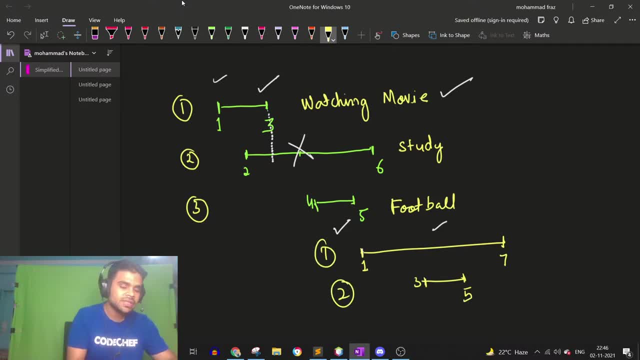 Which one will you select: Activity number 1 or activity number 2?? Tell me Which one will you select: Activity number 1 or activity number 2?? Meanwhile, I will tell you the question, which is new. The question is very simple. 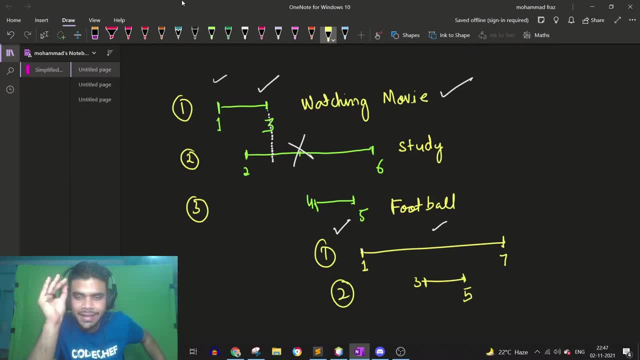 You are given a lot of activities. What is one activity? One activity is start time and end time. Basically, one activity is a pair of start time and end time, When that activity is starting and when that activity is ending. In this way, you are given multiple activities. 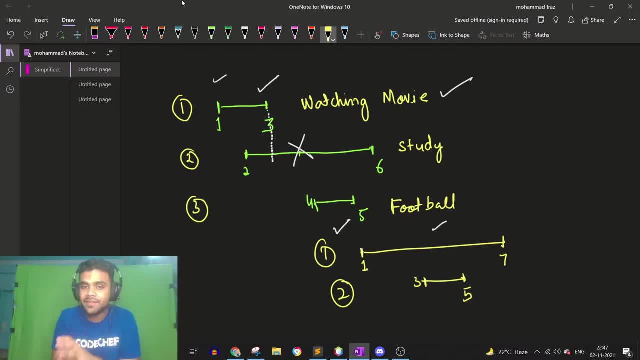 You have to select activities. Select as many activities as you can and maximize its number. Okay, Try to select as many as possible. When will there be a problem? Just don't have two overlapping. Okay, Two activities cannot be overlapping. This is the question. 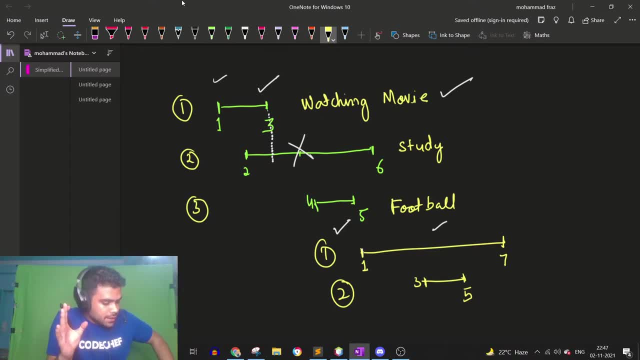 Very simple. Okay, Yes, Tanuj, you still don't understand. Tanuj, I have just explained to you. Implement that thing which I have explained. Please, who is spamming this? Please don't spam. Study. Study what we are studying. 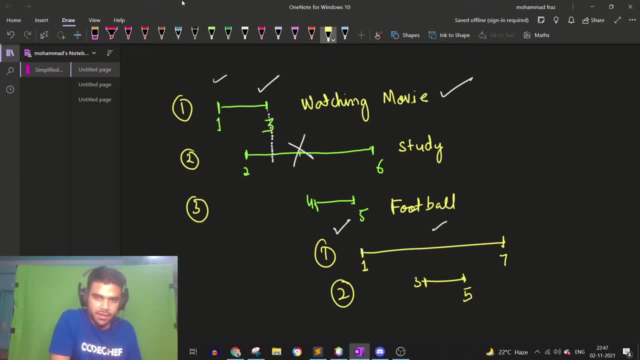 Okay, Later. ask your questions later. For now, learn what is being taught in front of you. It is not a very long class. Learn this thing with focus. Okay, So Tanuj still gave the wrong answer. Everyone else gave the correct answer. 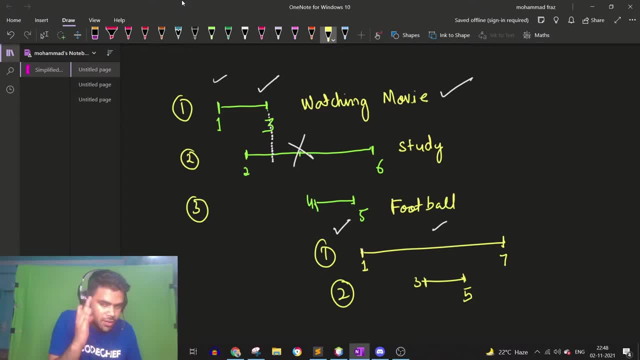 So I am happy for that. But, Tanuj, you still don't understand The activity which is ending earlier. See, it is not necessary. Why will I select it, Means? why will I select this activity? Why will I select this activity when this activity will leave me at 7 o'clock? 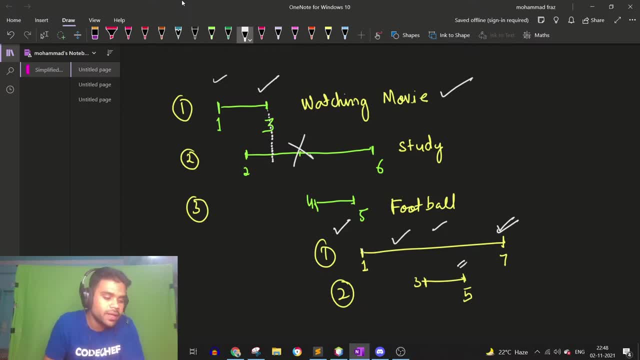 There is one activity which is leaving me at 5 o'clock, So I will select that. It is very simple: The activity which is leaving me earlier. I will select that. The activity is leaving at 5 o'clock, Got it? 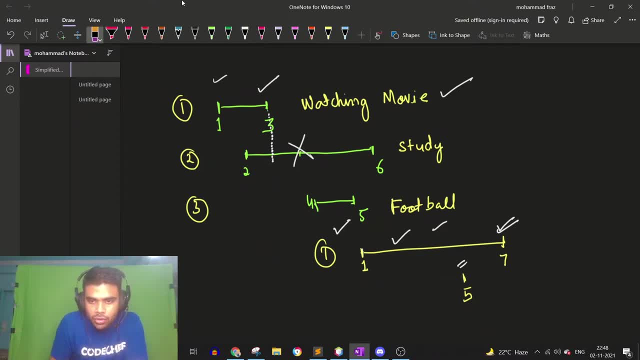 And if this was the case, If this was the case, The activity would have left us by 5 o'clock, And this would have started from somewhere here. It would have started from very early, And it would have left us earlier. Then as well, we would have selected this. 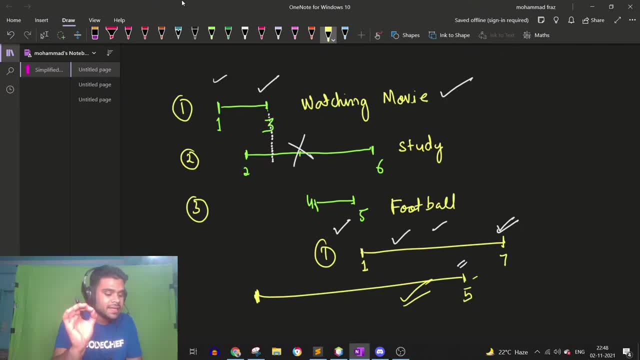 We don't have to see where the activity starts, we just have to see where the activity ends. So whichever activity is finishing first, we will be choosing that activity first. Got it Now. I hope everyone understood. So many people have already given me the answer to this. 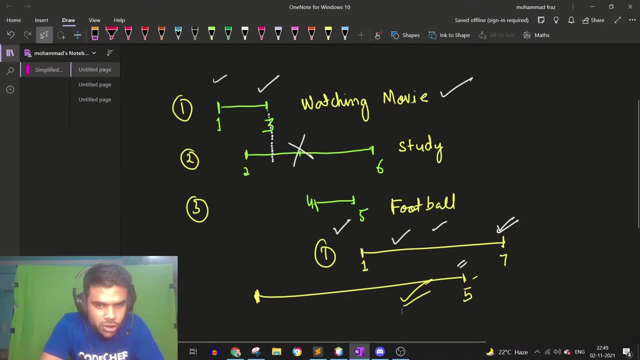 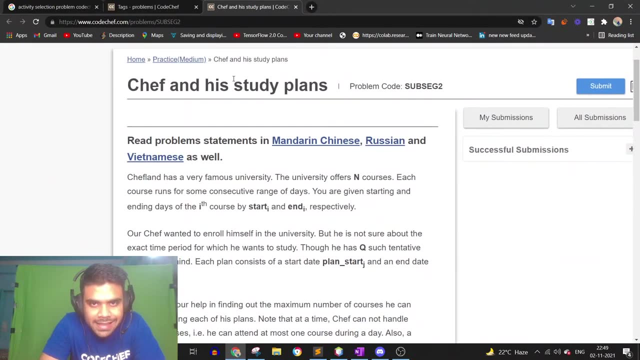 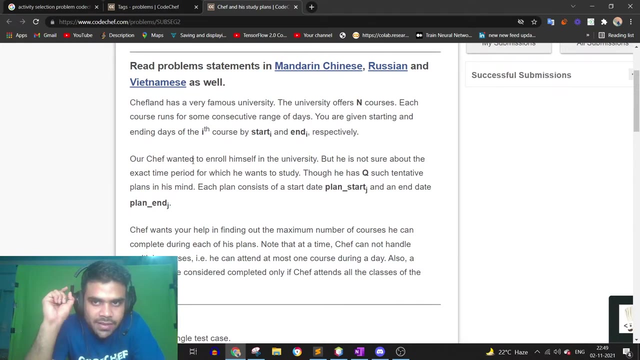 Let's read the question once. Let's read the question once. The question given on CodeChef: is it the same question? The question is: Chef and his study plans. Chefland has a very famous university. The university offers n number of courses. 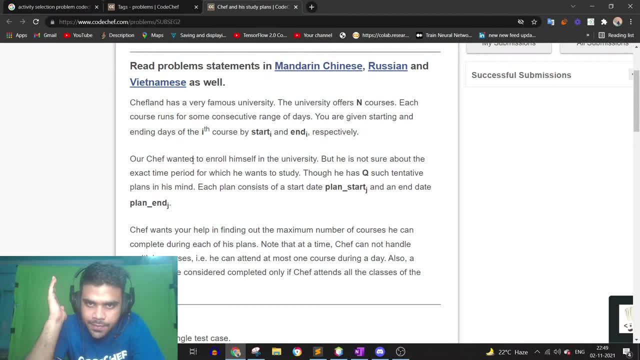 Each course runs for some consecutive range of days. You are given the start and the ending day of the i-th course by start i and end i. Basically, here, instead of time, days are given. No problem, it's the same question. 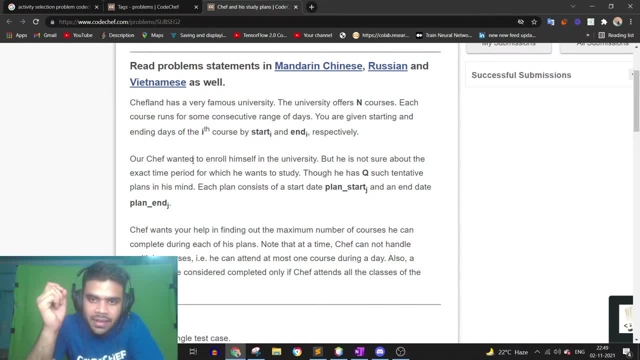 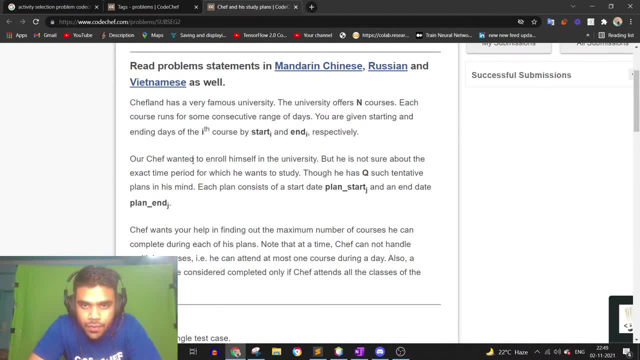 time period for which he wants to study. Though he has queued such tentative plans in his mind, Each plan consists of a start: Okay, Okay, Okay, Okay. Chef wants you to help in finding out the maximum number of courses he can complete during each of his plans. 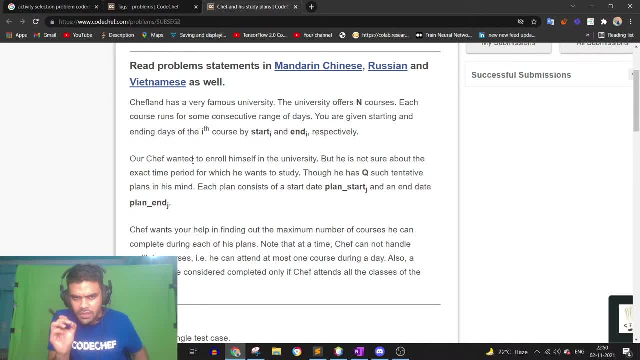 we have many plans given here. every plan has a start time and an end time. so we have to tell that, from this start time to this end time, how many courses can you cover? the question is same. it is little more advanced. there is no problem, I guess. 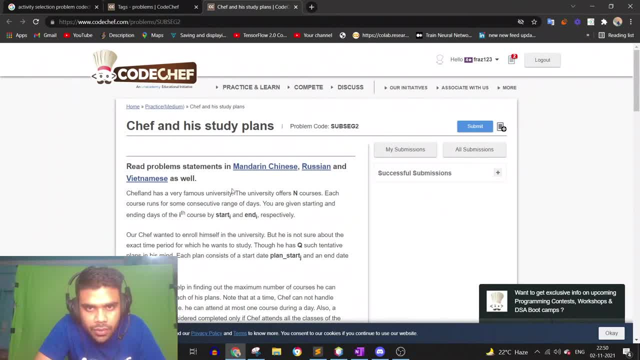 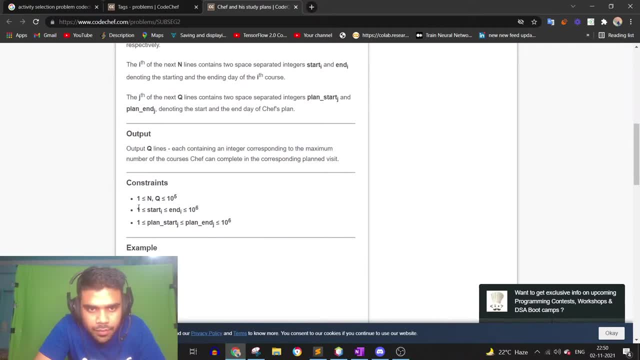 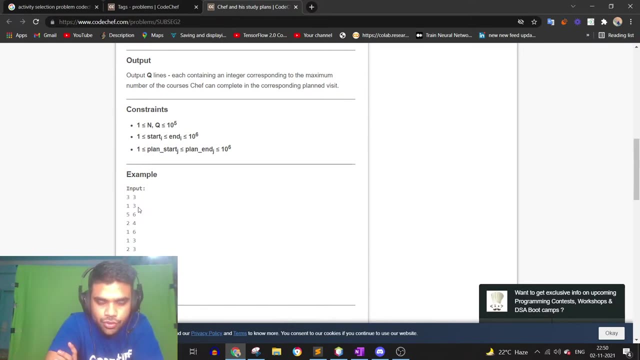 medium level? don't think so. it should not be medium level. is it really medium level? ok, ok, constraints are: 10 raised to the power 6, or how many queries? 10 raised to the power 6, 5 queries can be there. wow, alright, big O of N for that. 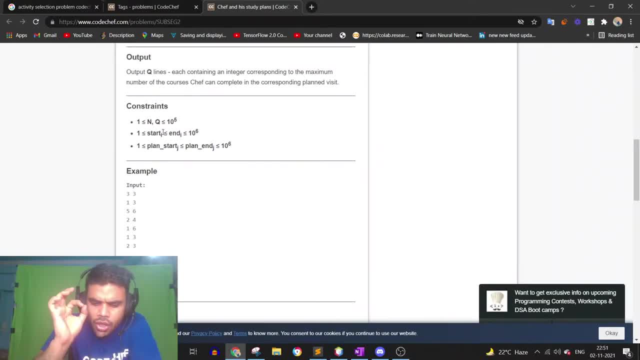 ok, ok, ok, ok, ok, the question is somewhat same, but here in the question you have to answer multiple queries. that is this is why constraints are too high. ok, it is 10 raised to the power 5. so Q- number of queries, and the N is also 10 raised to the power 5. 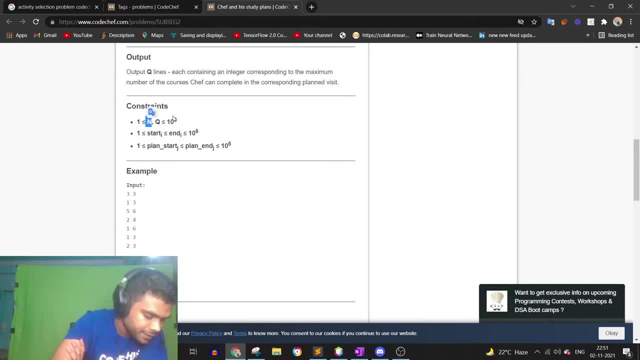 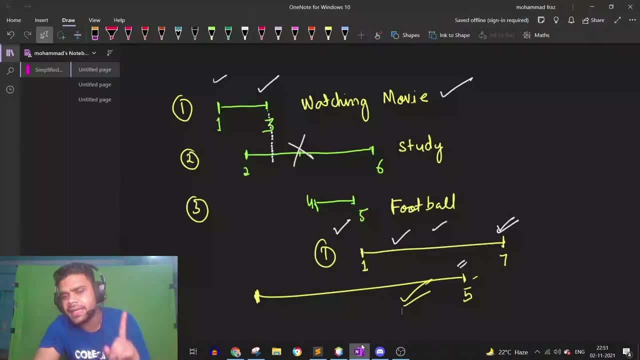 so here, 10 raised to the power, 10 will work if we square N. so it is going to be complicated. this will be a little complicated, but ok, what we were discussing, what we were discussing is only for one case. in one case it can be very easily. 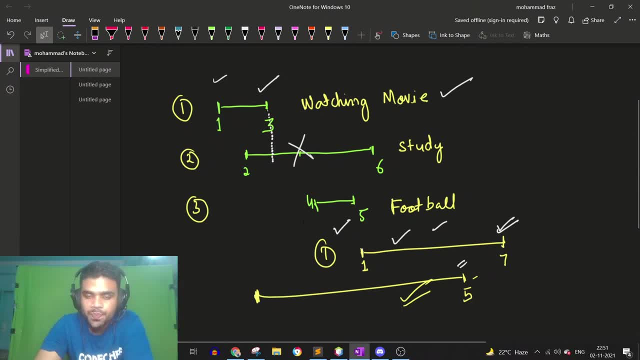 how can it be? sort them according to the end time. according to the end time, you have sorted them. after that, simply start picking the activities. ok, now, if we sort our example according to the end time, so it is going to be first of all which activity will come. 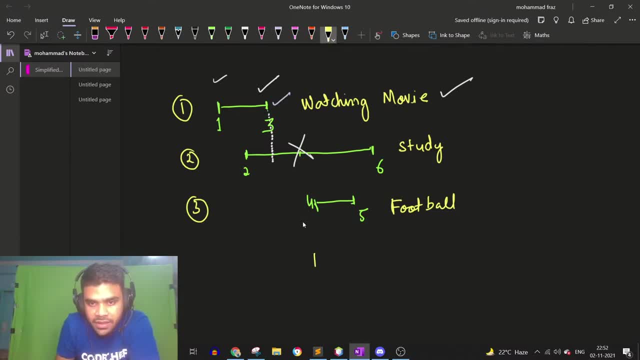 activity number 1 is going to be first. first of all, it is getting finished. activity 1 is going to be first. activity 3 is going to be the second one. activity 2 is going to be the yeah, activity 2 is going to be the third one. 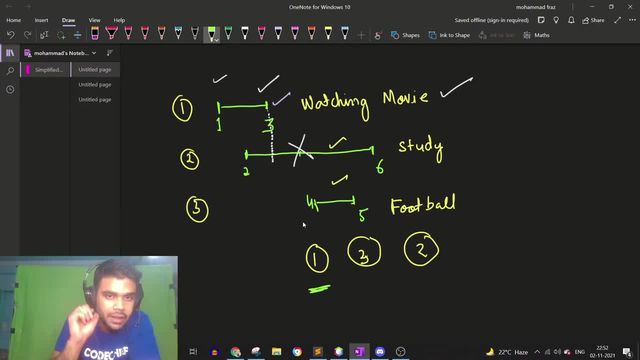 ok, so first of all, we will pick activity number 1. after picking activity number 1, we are not going to pick anything else till 3 o'clock. so till 3 o'clock, whatever will come, we are going to simply skip that. we will skip that. 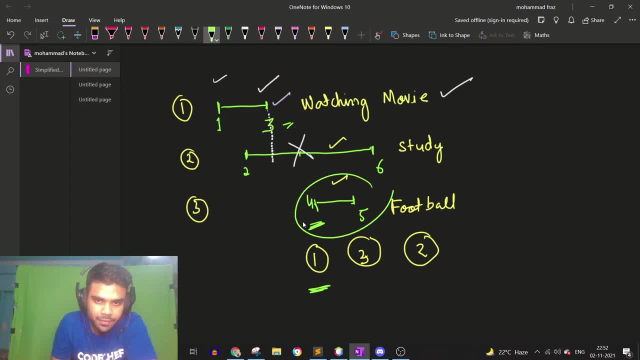 ok. after that we will select activity number 3. in total, we will be able to select 2 activities. ok. ok, we will move onto the next activity, which is again activity 3. we won't be able to see activity 3 if it will be activity 3. 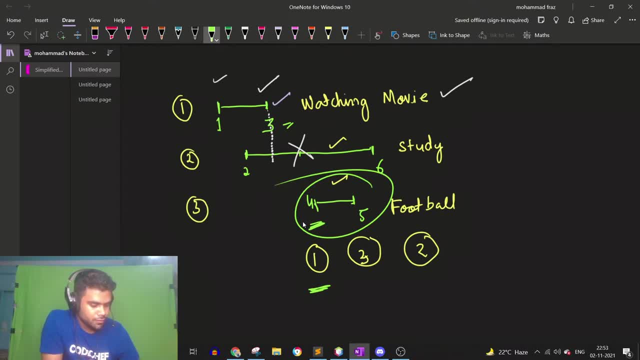 then etc. if it will be activity 3, then ofc. activity 3 will be cleaned. activity 3 will fill the activity. Yes, Got it Clear. Yes, sir, Nice. Okay, Siddhi, abhi tak, you didn't get the intuition. 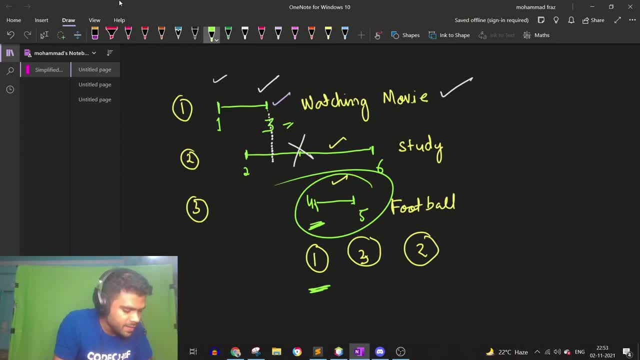 Nahi aaya, Tanuj ko bhi nahi aaya. We have to maximize the number of activities. Yes, we have to maximize the number of activities. Kyunke scene samajh nahi aaya Scene samajh. 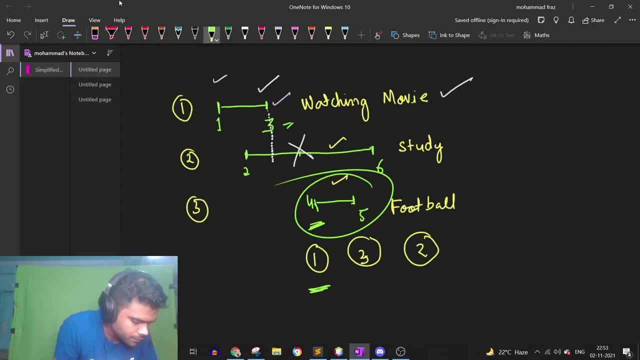 nahi aaya Thoda bahut. Ye Main to question nahi aaya samajh. Aap rewind karo, Mayank. Aap late join. kya tha apne to aap question nahi pata hai. Aap thoda se rewind karke. 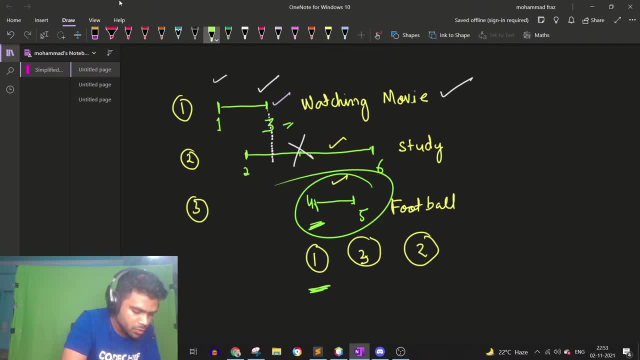 dekho. Okay, Chalo To. basically, I want to select the activity which is getting over earliest. Sabse pehle jo activity khatam ho jayegi mujhe wo select karna hai Activity ki length. 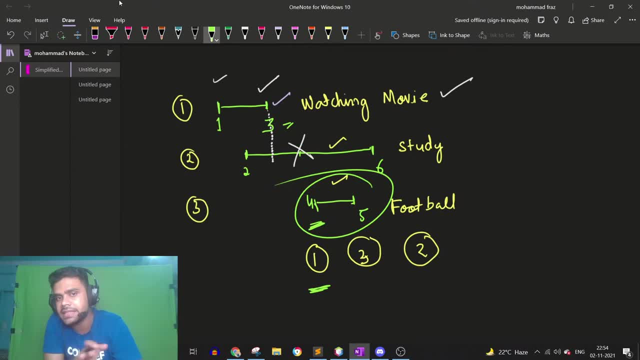 Se mujhe koi farak nahi padta, Kitni lambi activity Activity ke start time se kuch farak nahi padta Ki kya start time hai activity ka, Jo activity sabse pehle khatam ho riye. 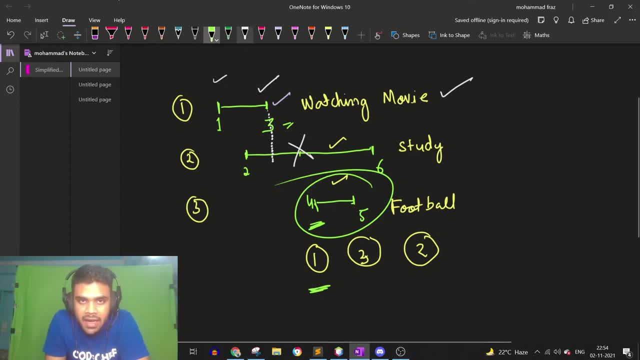 I have to select. that first Thik hai. Abhi, isi case mein aap dekhlo, Agar aap activity number one ko pehle select karoge. na Tabhi aap faide mein rahoge, Kyunke aap 3 pm ya. 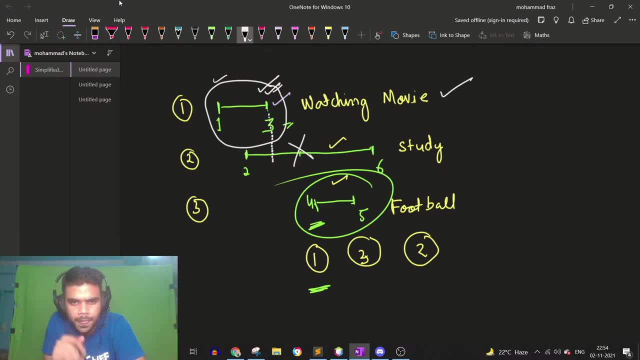 3 am. jo bhi hai. 3, 3 wajah aap log free ho. jaoge Sabse pehle Activity 2: select karli to 6 wajah free hoge. Samjhe Sabse pehle ham log free ho, na hai na. 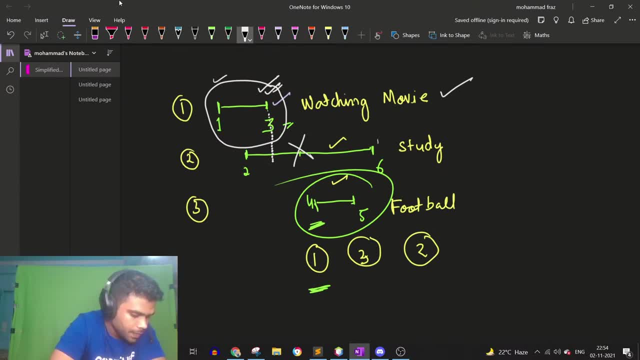 That is what we want, Got it. So sort it Inko sort karo according to the ending time and then start picking up the activities. Activities ko pick karna. start kar do Ek particular activity. agar aap logonay select kar li hai To dusri wali activity, jabhi select. 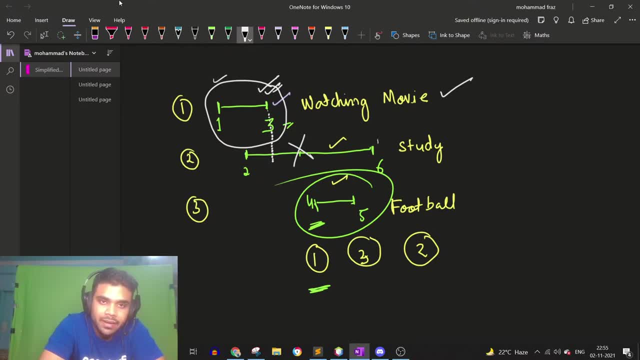 karoge, Jab dusri wali activity ka jo starting time hai, Wo pehli wali activity ke ending time se bada hoga. That is also the second condition. Got it Karke. dikhaye kya isko code. Do you want me? 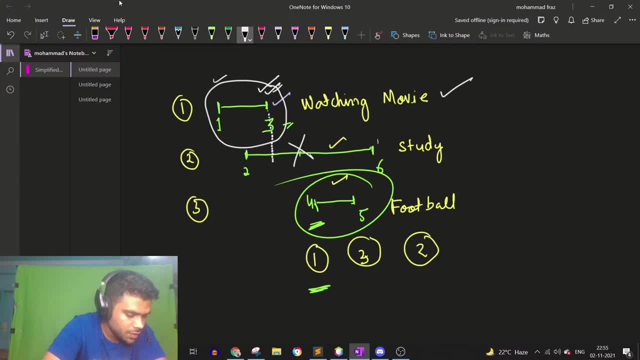 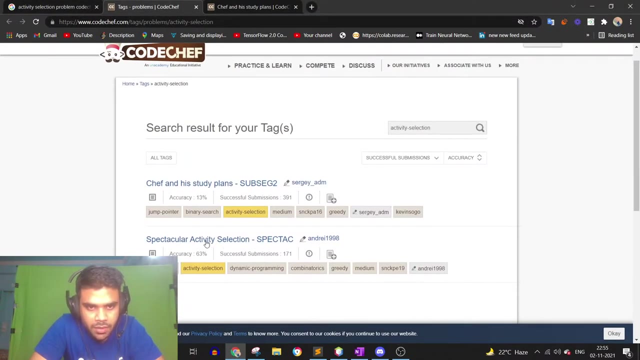 to code this. Kya aap isko code karwana chahte hain? Let me see, yaar. Hi codechef, mein advance wala question hume mil gaya activity selection ka. We didn't get the easy one, Spectacular. 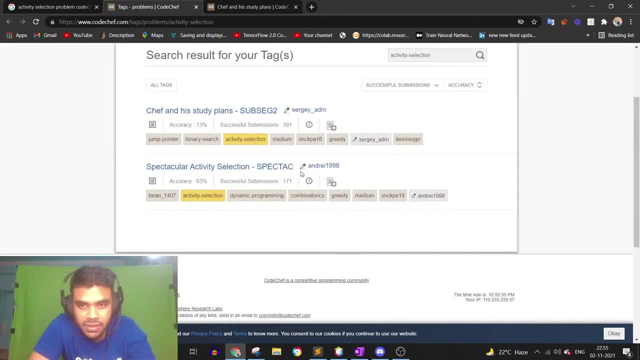 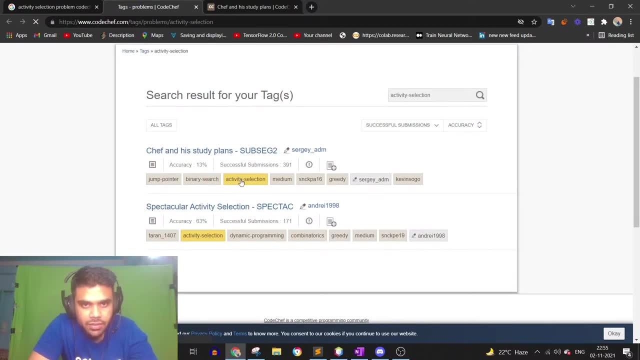 activity selection: Sif: 390 submissions hai. Iske aur bhi gama hai 171 submissions hai. Activity selection. Just want to search the tag Activity selection. Do hi hain yaar yaha par. I guess that simpler. 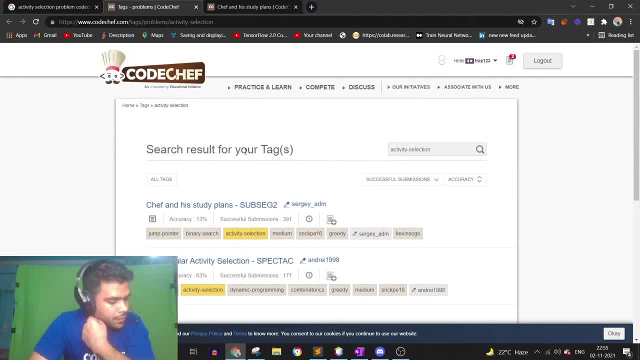 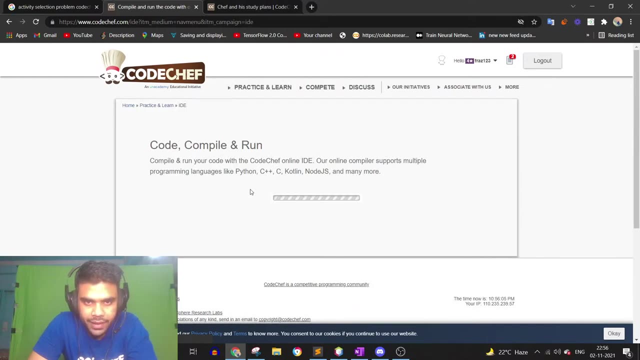 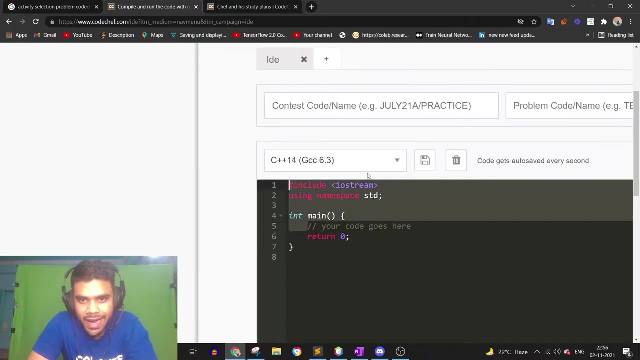 version is not here, But theek hai. We can still code that. Hum log isko code to kari sakte hain. So basically, let me go to the IDE. IDE pe chalte hain Codechef ke and let us try to code that. So I will be given an array. 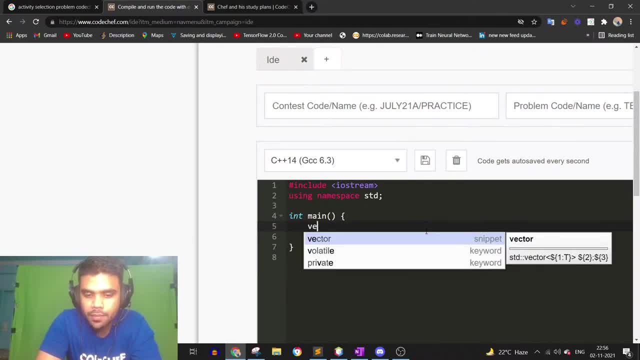 Ek array given hoga mujhe, Aur array mein kya hoga. Vector of pair of int, comma, int. Kehlo isko Yaar par. vector of vector. bol do. Vector of vector. isliye Kyunki isme start time aur. 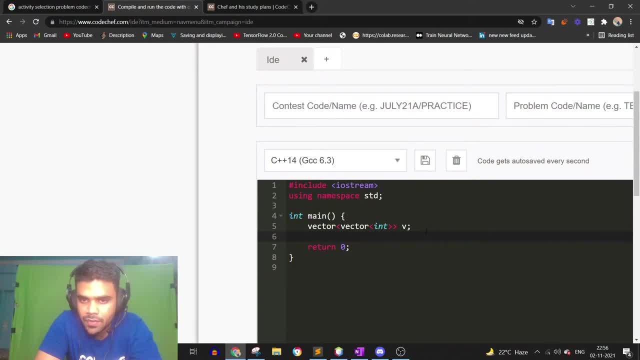 end time. dena hai, merku Hai na. I have to give the start time and end time. So I will give the start time and end time. So I will give the start time and end time. So I will give it as start time and end time. Let us say: 10 activity hain total, 10 nahin yani. 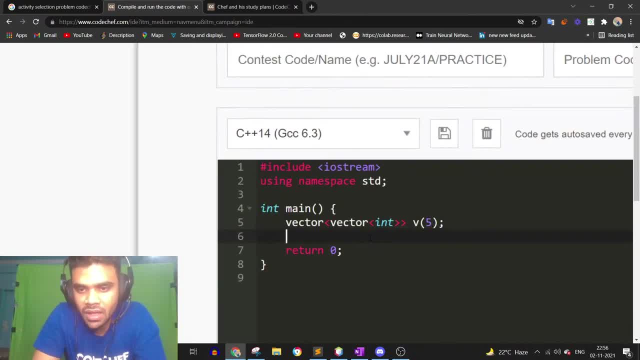 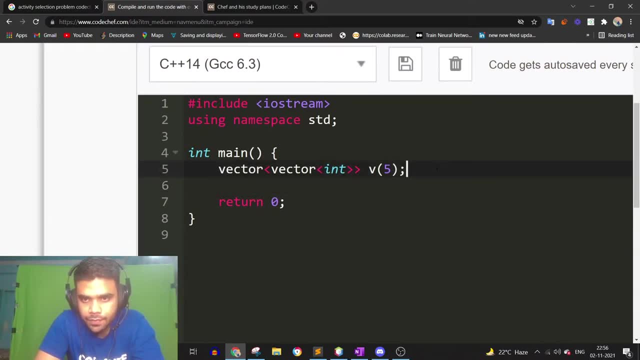 10 ton bohut saad honge. Let us say 5 activities hain total. There are total 5 number of activities, and first activity is starting at 1 and ending at abhi. hum apna hi example li lete hain. Agar hum upna hi example li lete hain. Yaha par main to hoon hai tene activityre hein First one, two, three Mani apna particuliers hai, apna particuliers hai tropal chein ne ek exemplo vee aap Luktaar ti long. 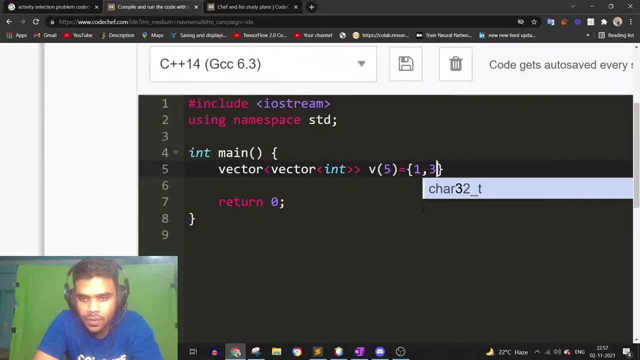 one se three tak hai pehli activity: One se three tak. Doosri activity hai aapki Do se chhe. teesri hai four se five Do se chhe aur four se five. These are the three activities. 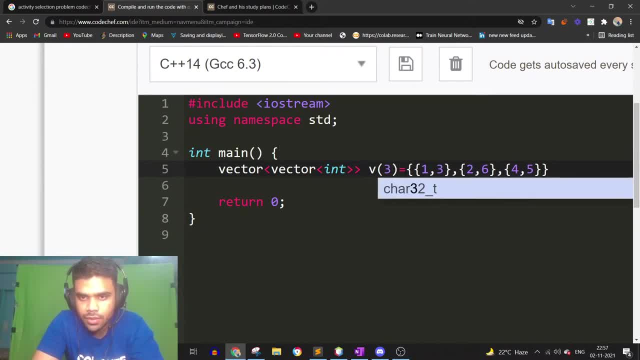 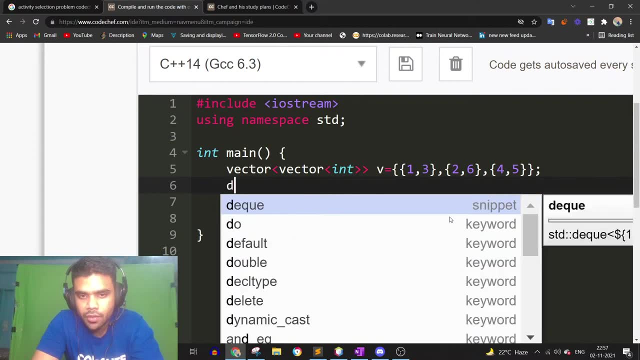 that we have Iska size bhi. hum teen le lete hain. koi rikkat nahi hai Ya directly aise bhi kar sakte hain. Uske baad hume kya karna hai? we have to sort it according to the. 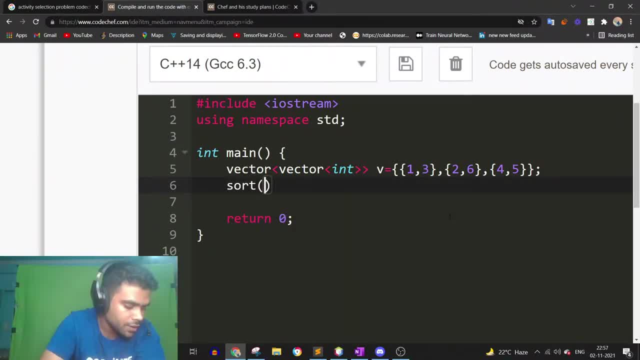 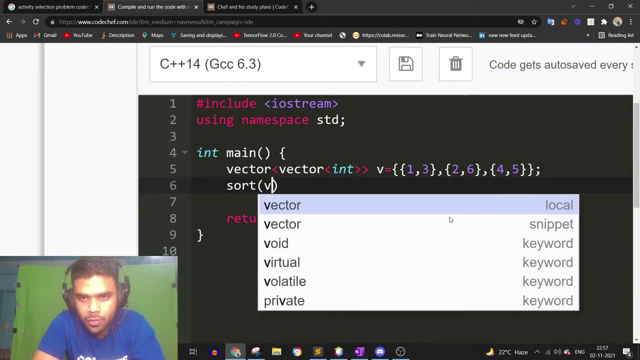 ending time, Activity ke khatam hone, ke time ke hesaab se inko sort karna hai. Pankaj, yaar, tumne class abhi join kiye late. Ab usme meri galti hai. batao Tum, kaya rahe ho ki mujhe. 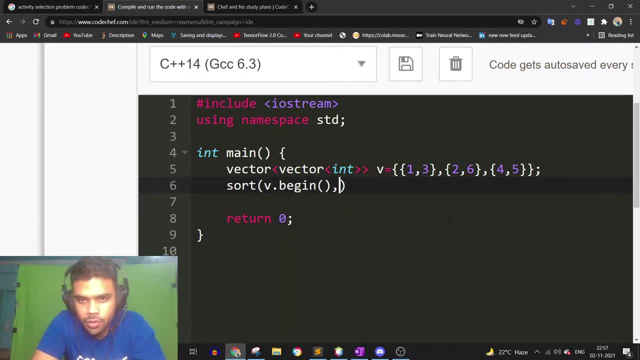 difficult lagra hai Abhi abhi class join kiye tumne. Tum chahate ho, mai dubhar se bada hu. Baaki log bhi hai. jino ne pehli se kar rakhie thi, Unke liye main dubhar repeat. 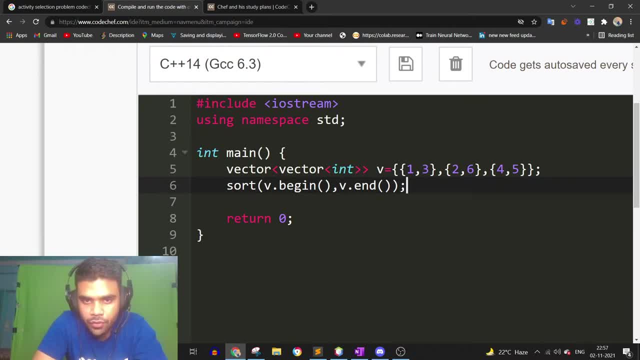 nahi karunga, Unka time waste hoga. Ab dubhar se dekh lo, rewind karke. You have an option. Sort karenge poori activity ko ending time ke hesaab se. Dekho, hum log jabhi sorting kar rahe hain na. 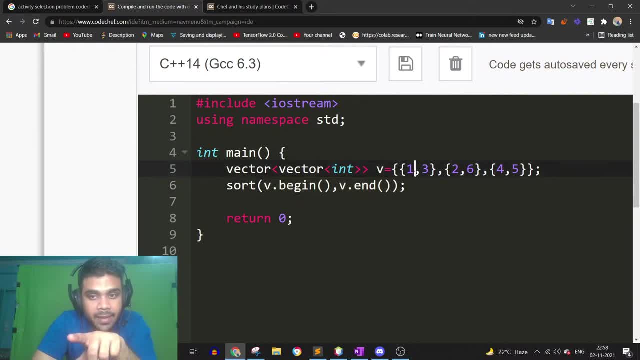 This sorting jo humne v peh laga diye abhi Ye starting time ke hesaab se sort kar dega saare activities ko. We have to sort it according to the ending time To isko nahin ek. comparator function- banana padega. Comparator function- banana padega- cmp. Let me create a function. 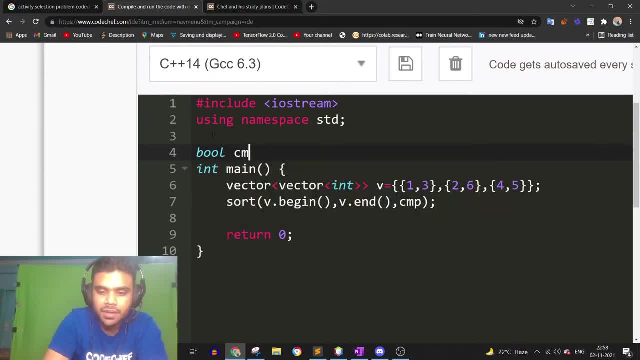 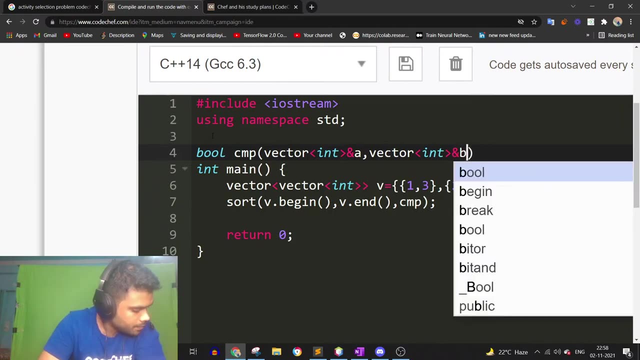 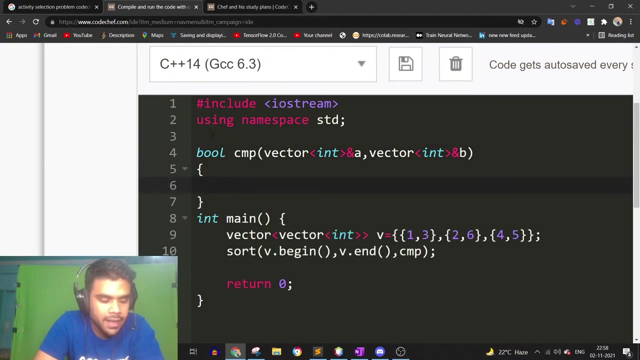 Boolean type ka function banate hain, Ek comparator iska naam hai. This function is going to take two arguments. The first one is a vector of integer a, The second one is a vector of integer b, As ke baad humne sorting karni hai. according to the 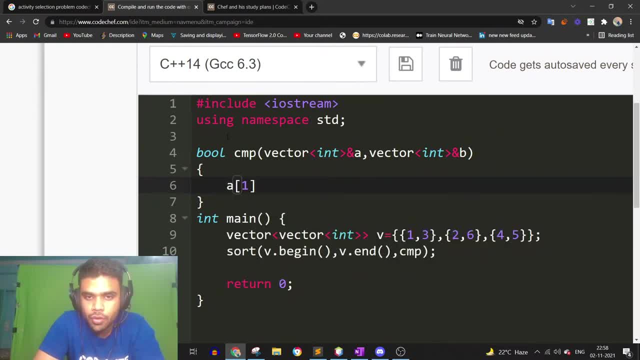 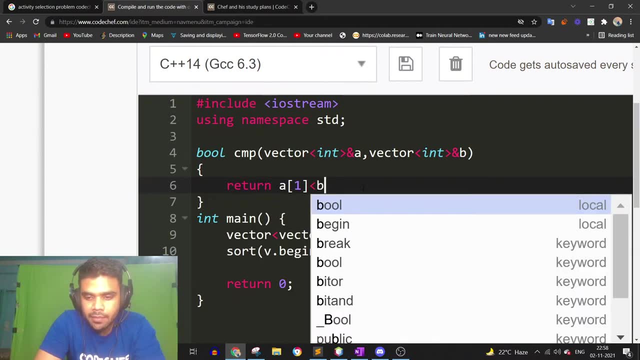 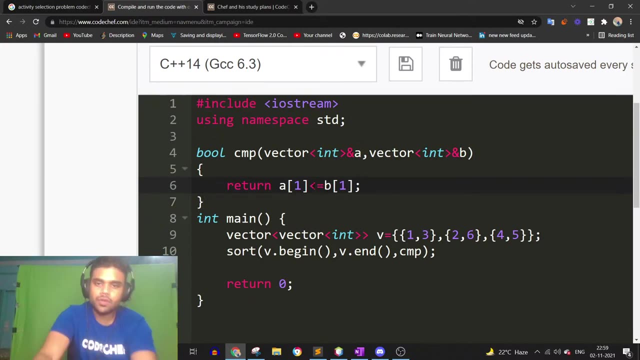 ending time to jo a hai uska 1 aur jo b hai uska 1: uske sab sorting karni hai. So if return, if a ka 1 is smaller than b ka 1. Let's keep it as smaller than or equal to. so this is our comparator, according to the. 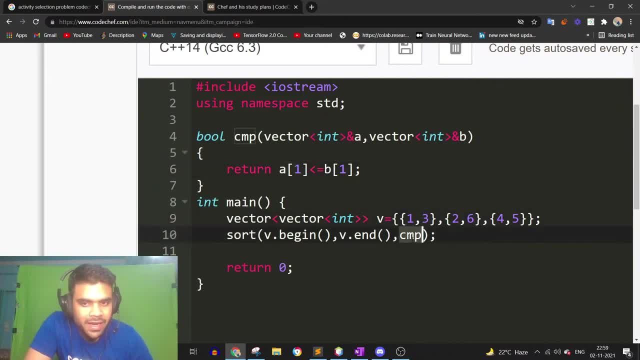 second argument, which is on index 1,. actually, two things will be passed in the comparator. first thing will be this vector and second thing will be that vector which is being compared. two vectors will be passed. actually, this is a vector of vector. if this was a vector, 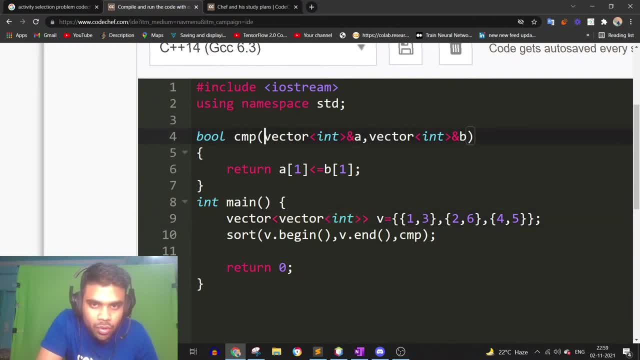 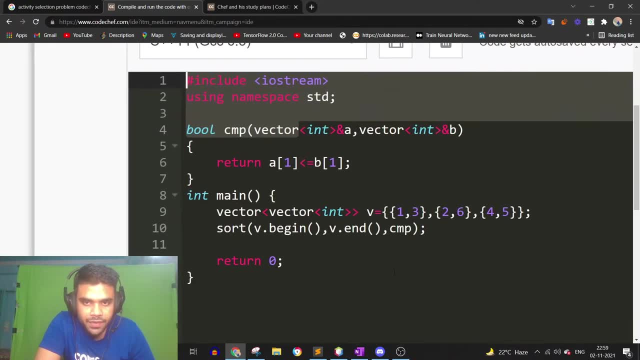 of type int, then in the comparator we would have taken int a, int b, but this is a vector of vector. so as an argument we will have to take vector of vector in the comparator, because there are a lot of vectors in this vector. so we have to compare vectors to sort. 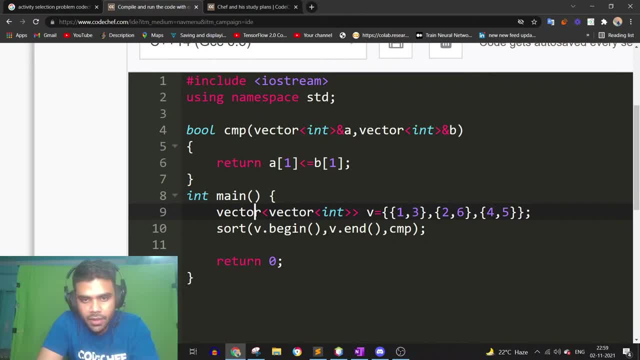 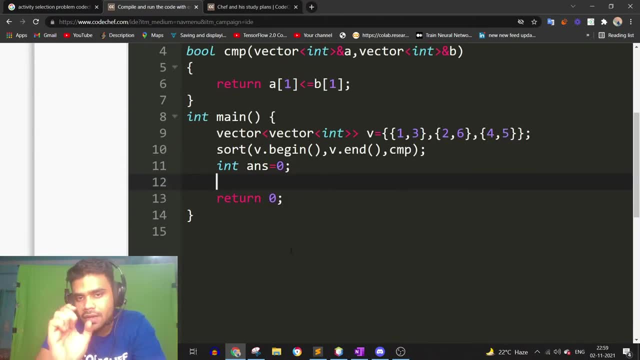 this after sorting: after sorting according to the ending time, we have kept an int answer which will be 0.. After sorting, we have kept an int answer which will be 0.. After sorting, we will go to all the activities. for int i is equal to 0,. i is smaller than. 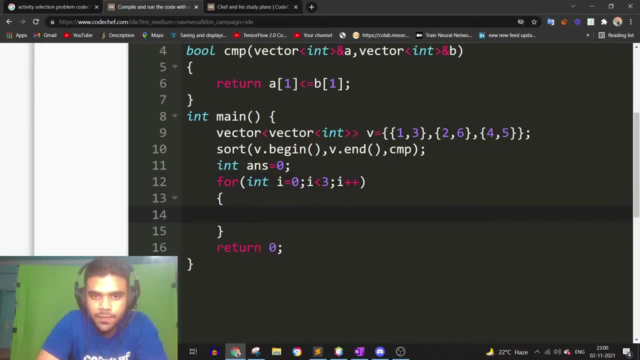 3, i++. we will go to all the activities and we will be selecting the activities. okay, One particular activity. when you can pick when you will be free. if you are free, then only you can pick a particular activity, okay. 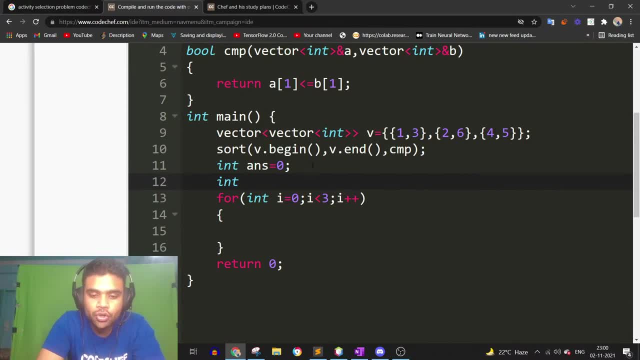 So now let's see when we will be free. initially we will free at. let's write it free at: initially we are free at 0,. okay, Initially we are free at 0,. so if free at this time is smaller than or equal to the. 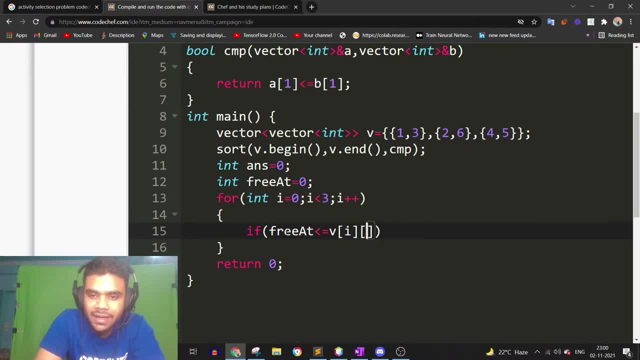 starting time of the current activity. ie v of i's starting time. ie v of i of 0,. if your current activity's starting time, your free time, will be less than the starting time of the current activity, then only you will be able to pick the current activity. 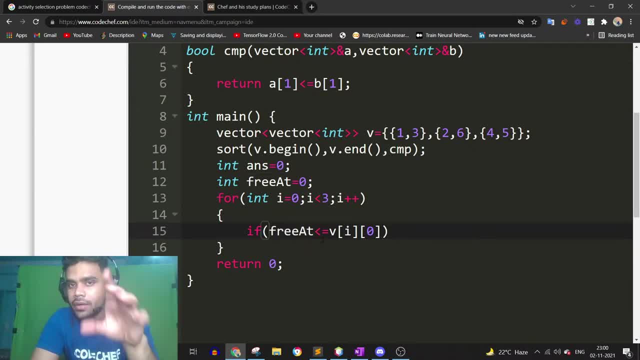 otherwise there is an overlap. Let us say you are going to be free at 3 o'clock. you have selected an activity that will free you at 3 o'clock. then you will ignore all the jobs that will come before 3 o'clock. 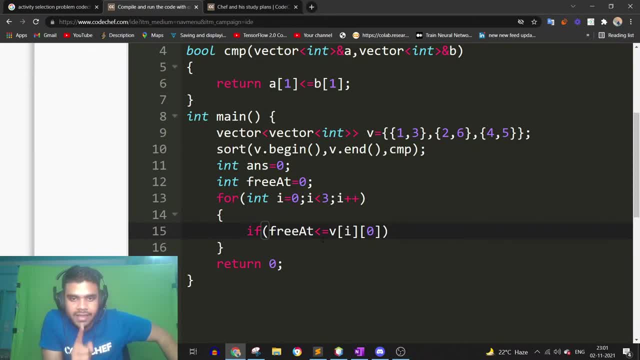 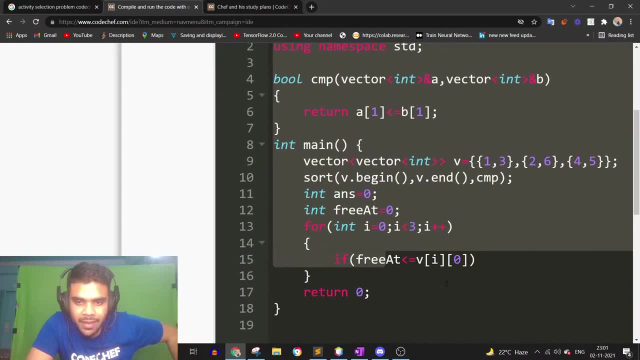 right, You will be able to pick the job after 3 o'clock. that is why, if the free time is smaller than or equal to the ie, if it is already free, then only you will select it. okay, After selecting what will happen. 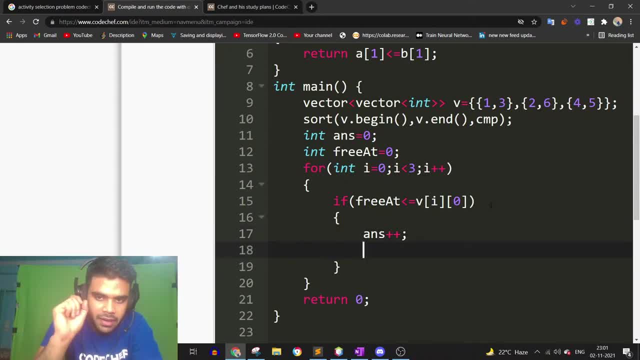 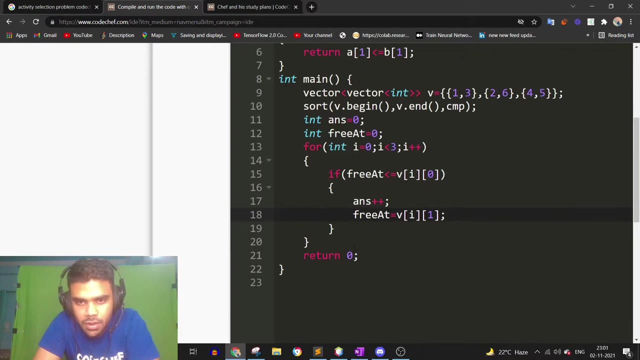 The answer will increase. you have picked the activity. after that, free time will change. free time will change Now, if you have selected the activity that you are starting to do, the ending time of that activity is going to be the free time. this will be your free time, okay. 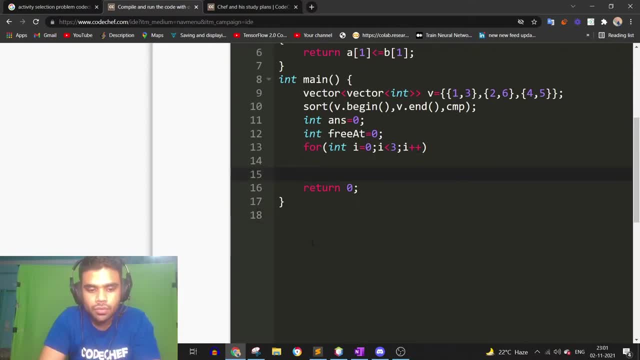 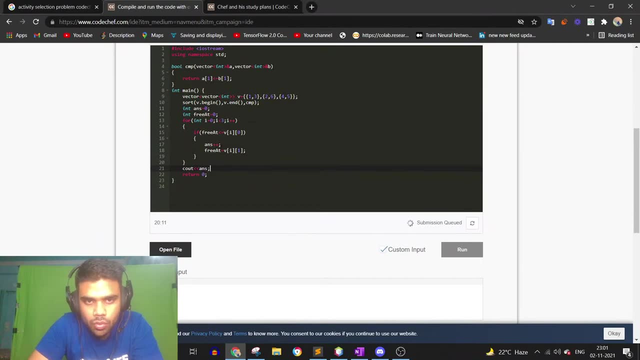 For the next time. By selecting all the activities like this, you will just see out the answer. Let us see how many activities we can select in our case. We have seen in our example that we were able to select 3 number of activities. 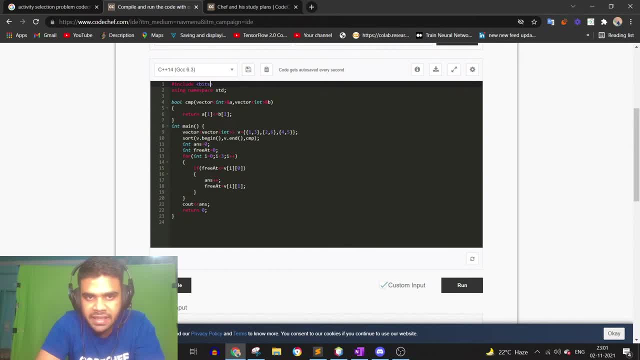 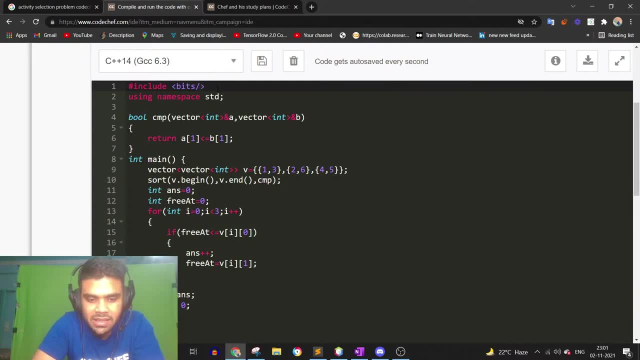 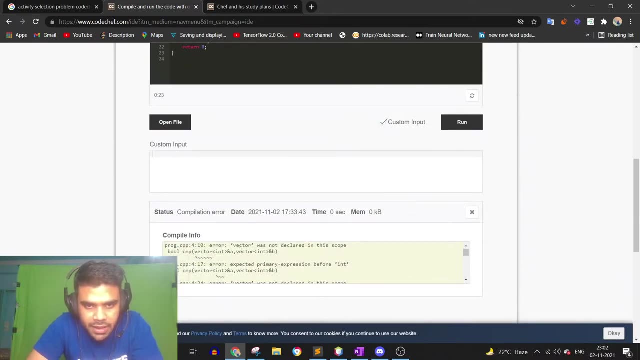 We have not changed the address here: Bits. we are using sort here. we are using vectors here. that is why we have to include here: hash includes bits slash, stdc++, dot h. Obviously the error will come in the vectors only. 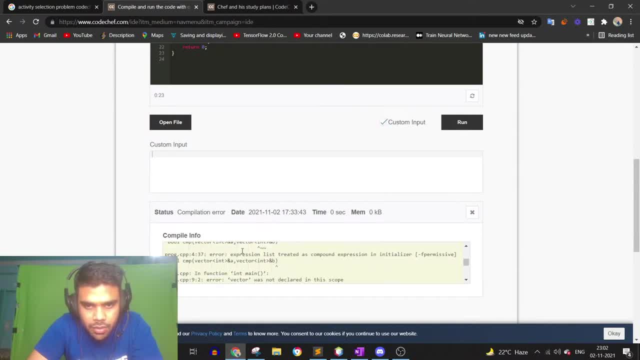 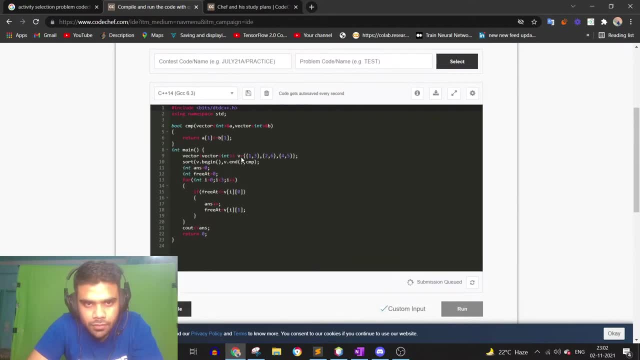 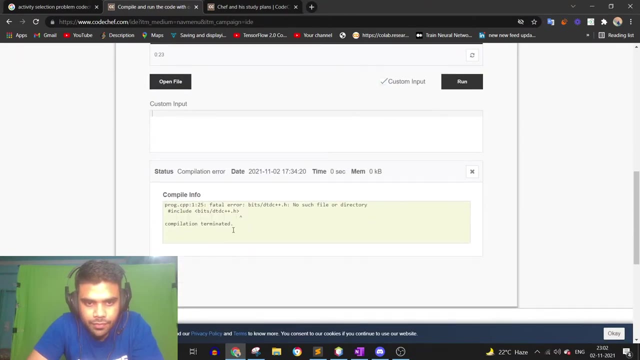 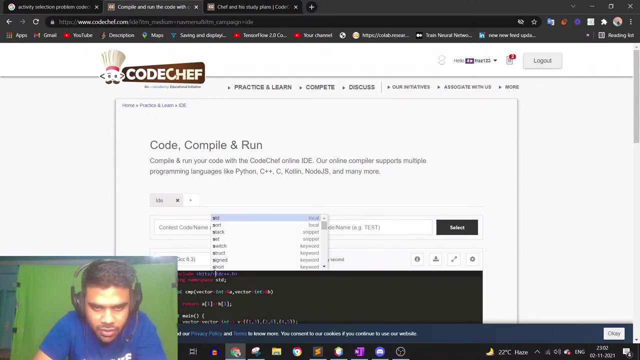 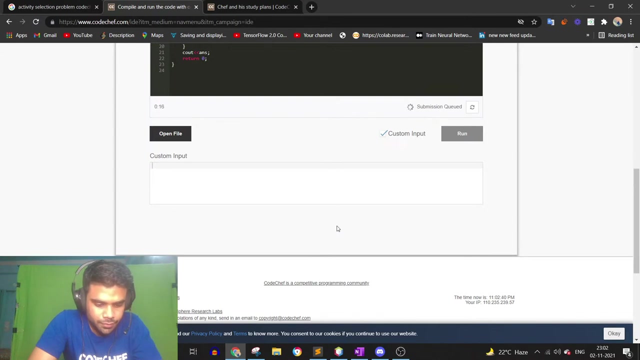 Vector not declared in the scope. Vector was not declared in the scope. Sort was not declared in the scope. Sort was not declared in the scope. It won't come because we have added the hash include file bits, Bits, slash. Our output is correct. Our output is 2.. 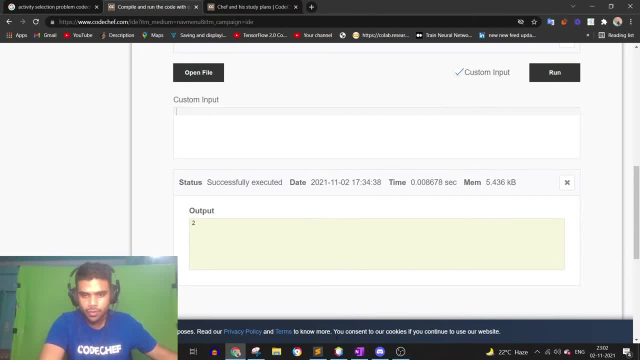 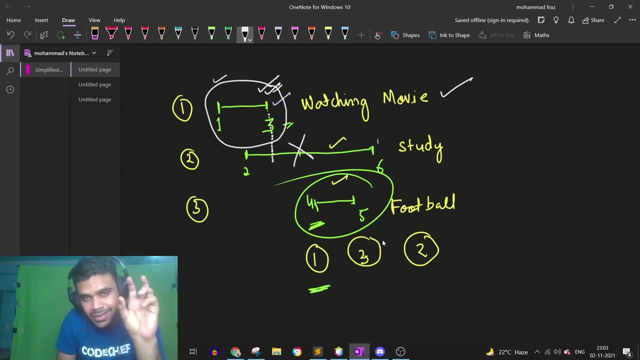 See, our output is correct. Let's take one more example. Let me take one more example. Let's modify this. Let's say: there is one more activity which is coming between 3 and 4.. There is one more activity which starts from 3 and ends at 4.. 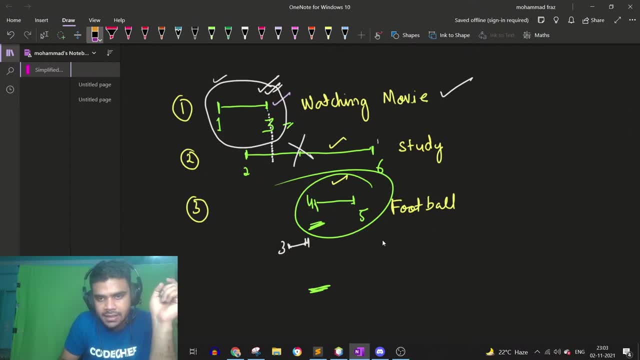 You guys tell me what should be the answer in this case. What should be the answer? And I will take one more activity, One more activity which starts from 5 and ends at 6. We have to add 5 and 6.. 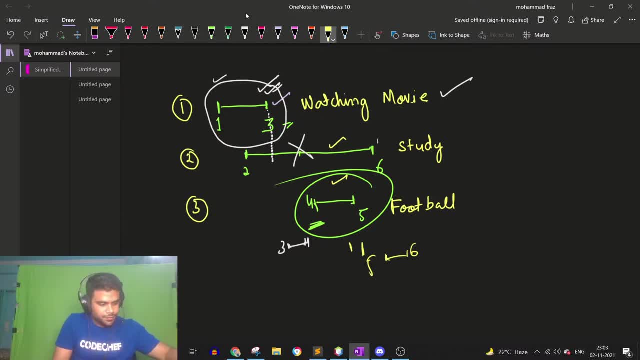 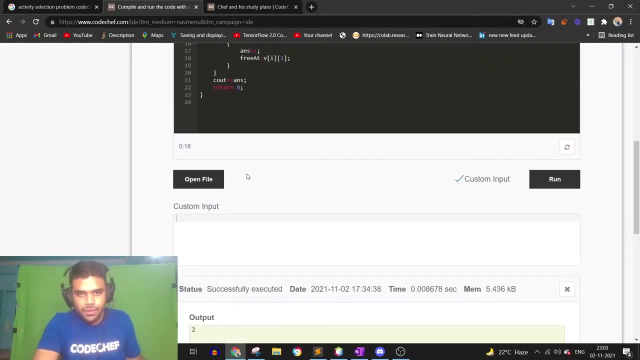 We have to add 3 and 4.. Tell me what should be the answer in this case: 3.. Yes, 3 will be the answer, Because this will also be selected. 3 will be the answer, Because this will also be selected. 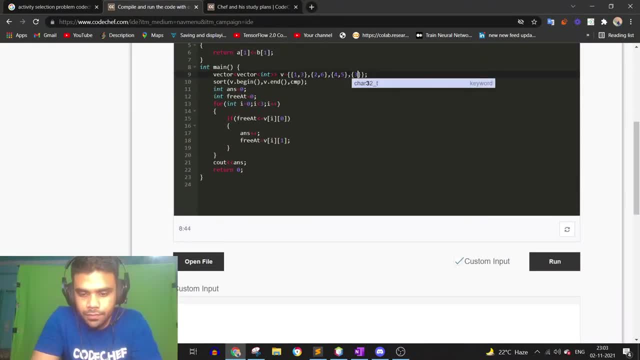 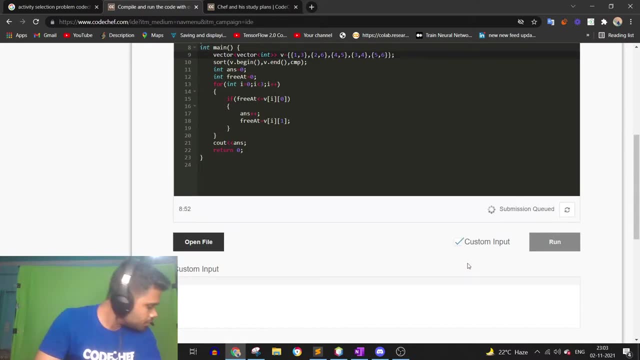 3 to 4.. We will do one more, And we will do one more: 5 to 6.. 5 to 6 will be selected. 5 to 6 will also be selected. 4 will be the answer. 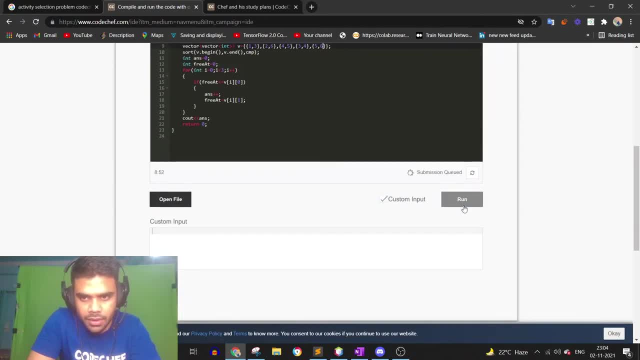 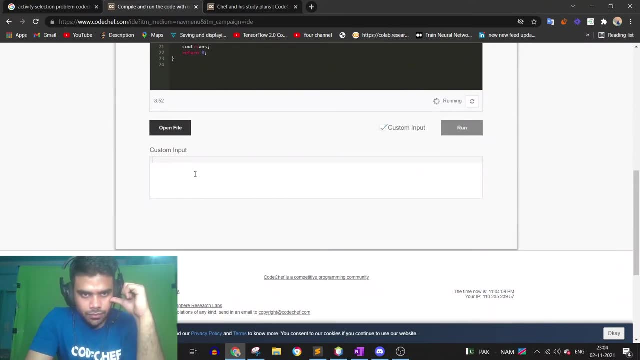 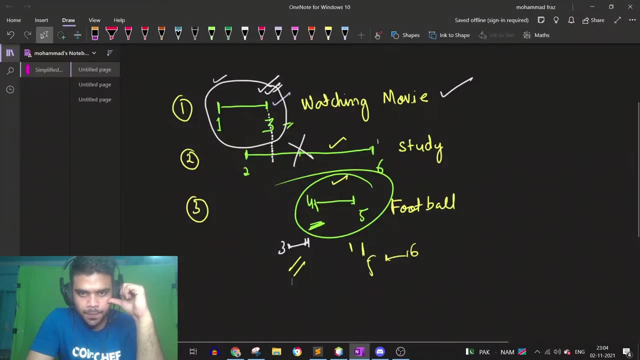 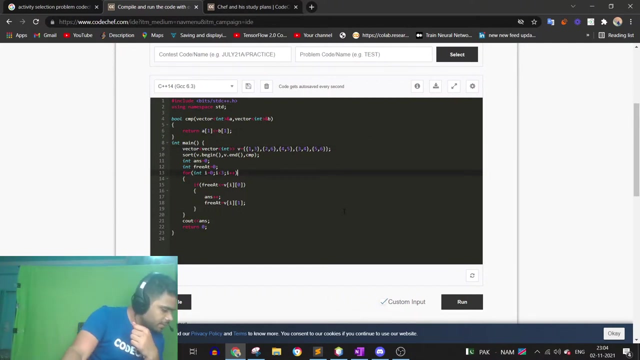 One second. How is the answer 3 coming? Answer 3 is coming. 5 to 6 will also be selected. 5 to 6 will also be selected. Why 5 to 6 should be selected? 5 to 6 activity should also be selected. 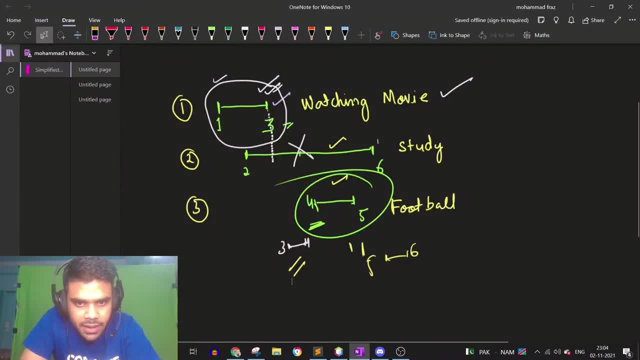 Why is it giving me 3 as the answer? 1 to 3.. Continue trying 1 to 3. And we will complete 2 to 3.. Okay, Ok, After that there should be option 3 to 4.. 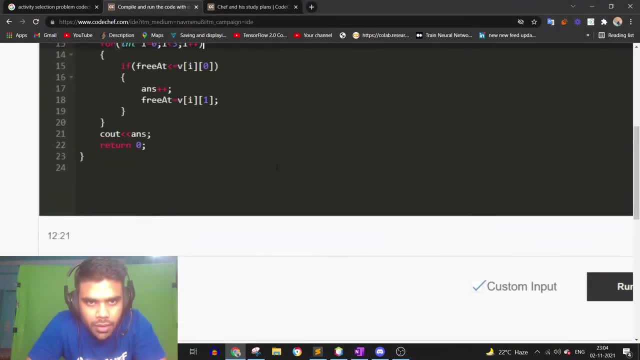 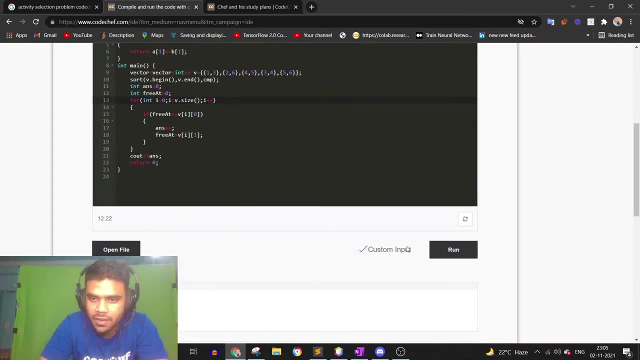 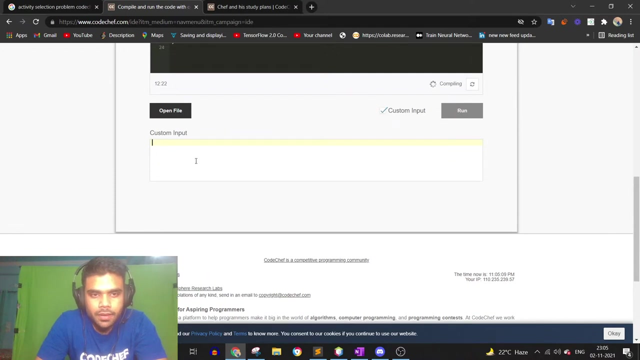 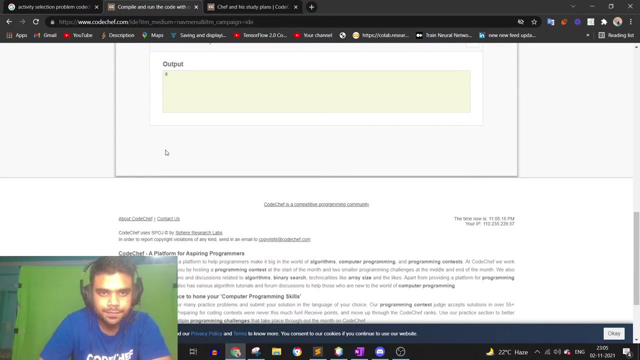 After option 3 to 4, option 4 to 5 should be selected, And option 4 to 5, there should be option 5 to 6.. Oh, I have added 3.. Sorry, Now we will get 4 answers. we are getting 4 as the answer, okay. 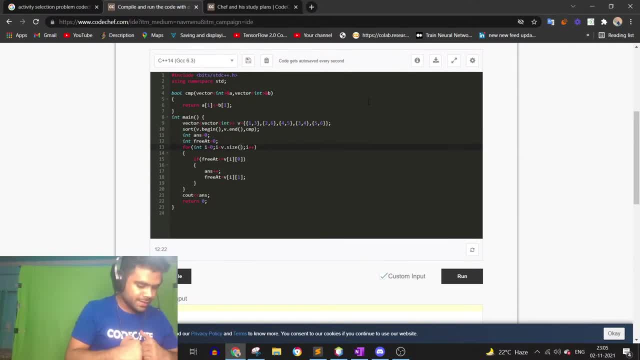 Did you understand? Hmm, It's good. it's good, Less than 3 dollars. Thanks a lot. Tell me, is it clear to you guys? Is the intuition clear behind this? How is it working? I hope everything is clear now. 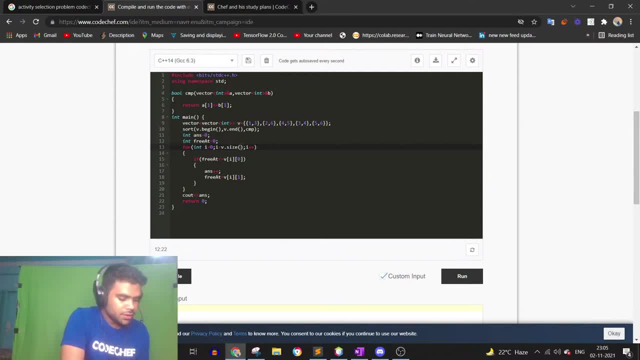 Yes, okay, nice, nice okay. Chandan Devrath, Siddhi Shivansh. okay, okay, okay, okay, okay, okay. Praval, very good, If everyone understands. please like the video. 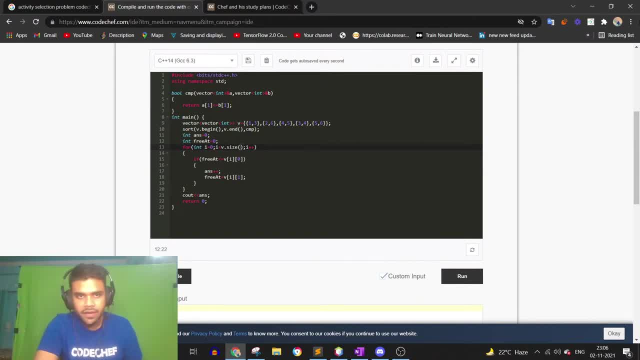 Okay, Now let us solve. let us look at one more problem. okay, Let's see one more problem. It's a little bit advanced, Not much, it's a little bit advanced. Let me take out the problem statement, Just having a look at. okay, okay. 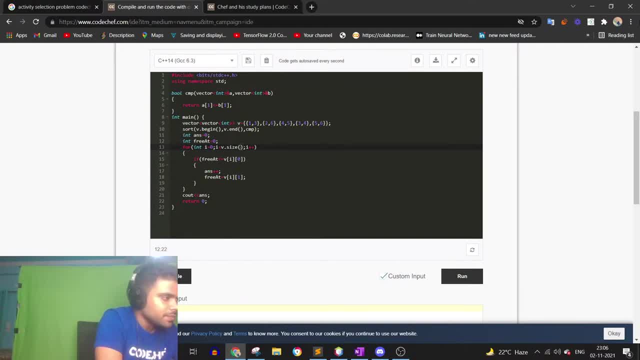 We have a few days today to do the activity activity selection, so let me take that problem here. Hmm, activity selection with profit. What we just saw that was activity selection: Maximum number of activities that you can select. Activity selection or job scheduling, whatever it is. 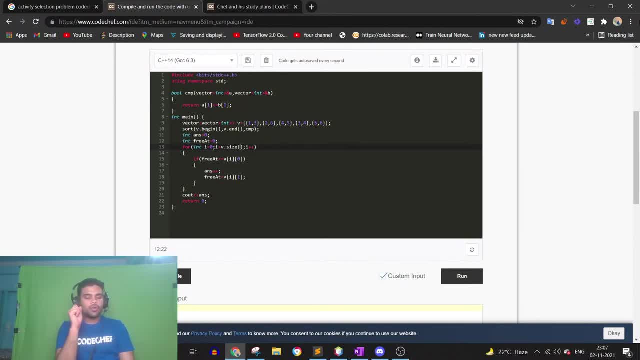 So now I have one more problem. In that problem, what you have to do is you will be given the start time of the activity. You will be given the end time of it. Along with that, you will be given how much profit you will get by doing that activity. 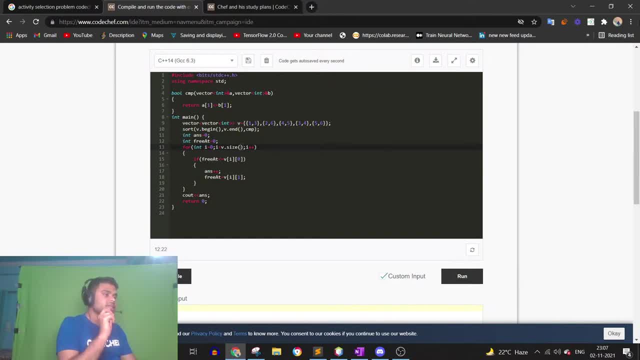 And now you have to maximize the profit. You have to maximize the profit, We have to maximize the profit. Tell me, How will we do it? We have given 3 things. It is buffering. I guess it's not buffering. It is not buffering. 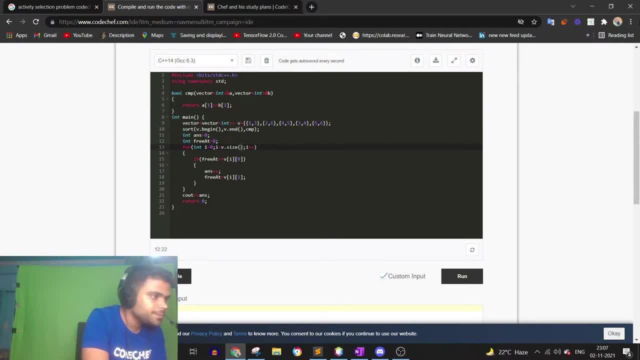 Is the buffer is getting done? No, Okay, By the end of the day, in the end of the day, it is a buffer, We have to keep it. keep it Here. a third parameter has been added, that is the profit. 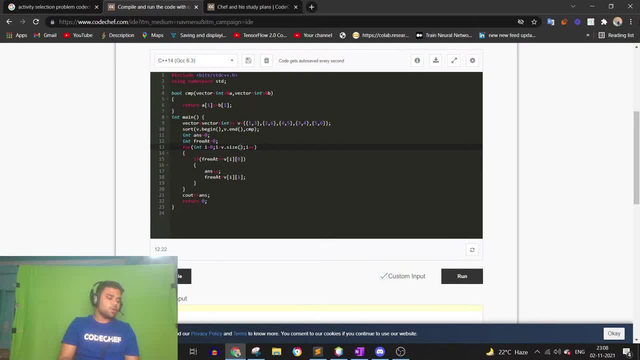 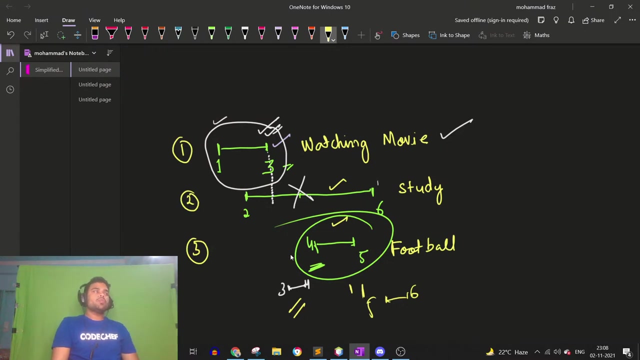 Every activity has a profit added to it. So tell me how are we going to calculate it? Somebody is saying: sort profit in descending order, then select. Basically, what he is saying is that sort profit in descending order and select the activity. So assume that this activity is giving you 100 profit. 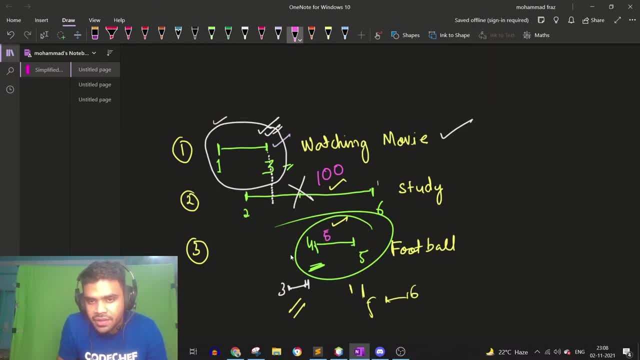 This activity is giving you 100 profit. This activity is giving you 50 profit, This activity is giving you 20 profit, This activity is giving you 10 profit And this activity is giving you 30 profit. Which activity will give you the most profit? 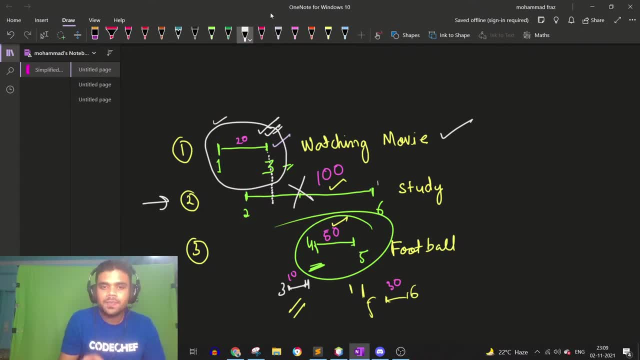 The most profit will be given to you by activity number 2.. But if you select activity number 2, then you will not be able to select 1,, 2,, 4, 5.. You will not be able to select anyone. 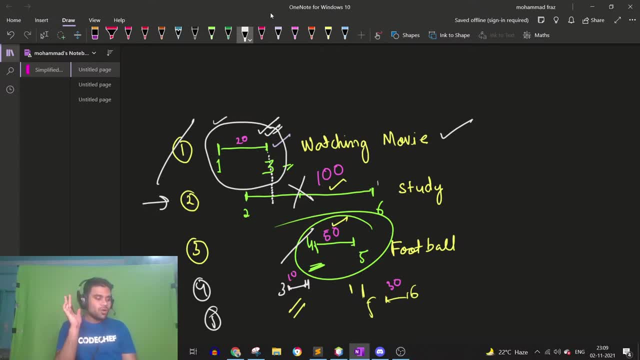 You will not be able to select the activity number 2 alone, And because of that, you will only get a profit of 100.. You will only get a profit of 100.. If you don't do this, then how much will you get? 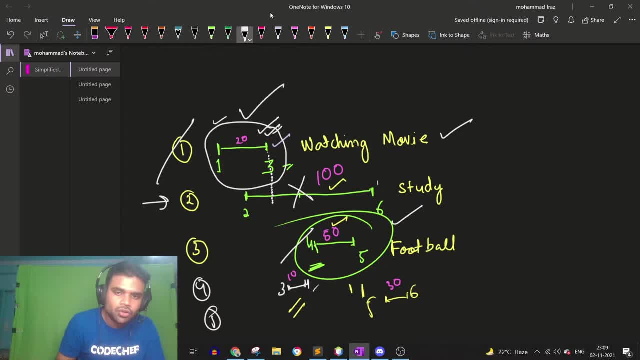 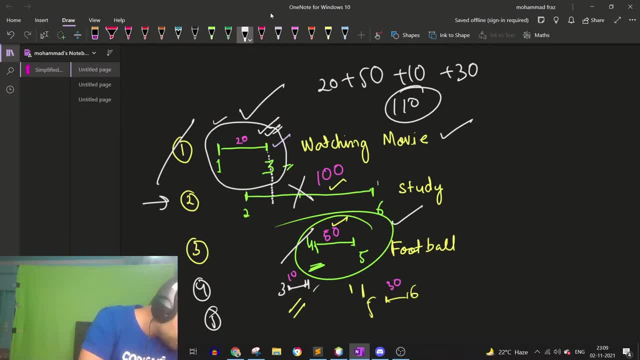 So that is wrong. That is wrong. Okay, Praval, We will keep the highest profit slot. Prioritize activities which give more profit. Wrong See, this will happen after that. Profit divided by profit slash time sorting: Profit slash time sorting: No. 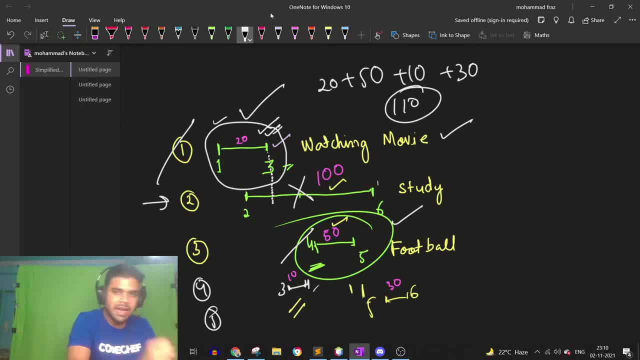 In the comparator function sort according to ending time and profit. Sort according to ending time and profit Or sort according to your profit. What is this combination? What is this combination of ending time and profit? You want to multiply them. add them together. 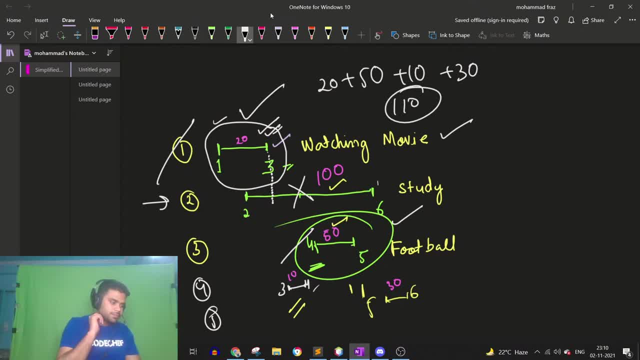 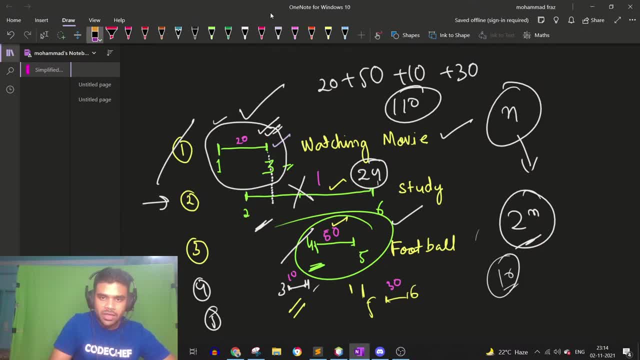 lets make it 105. let me make this 105. then its maximum profit per hour will be more than 25 and this activity will be selected first. but if you select this, then you will not be able to select other activity, which is wrong. you cannot maximize the profit. 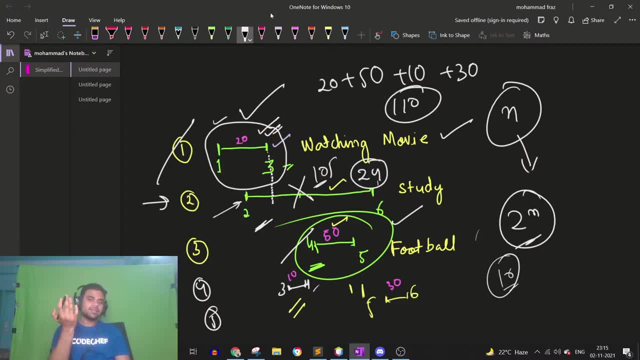 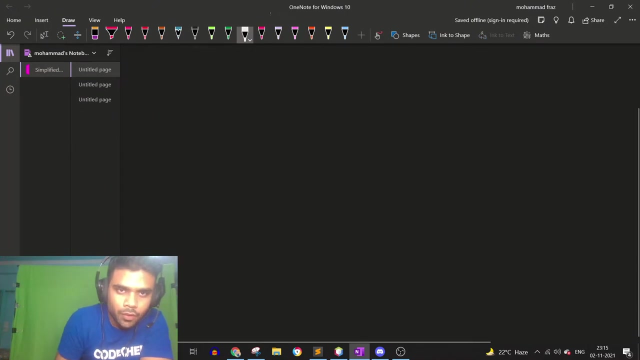 if you prioritize them according to the maximum profit per hour, we will select the activity according to the end time and take maximum value of activity which is giving maximum profit. let us start discussing it. we will start discussing it. we have activities and their profit got it. activity 1: 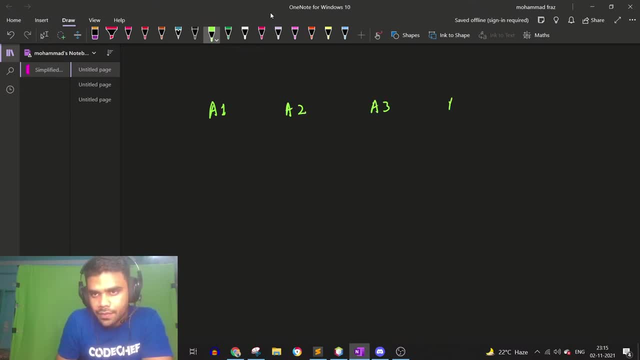 activity 2. activity 3. activity 4: activity 5: there are several activities which we have. each of these activities is having a start time, end time and a profit. got it so and assume that, according to the end time, we have sorted them so that we can select maximum number of activities. 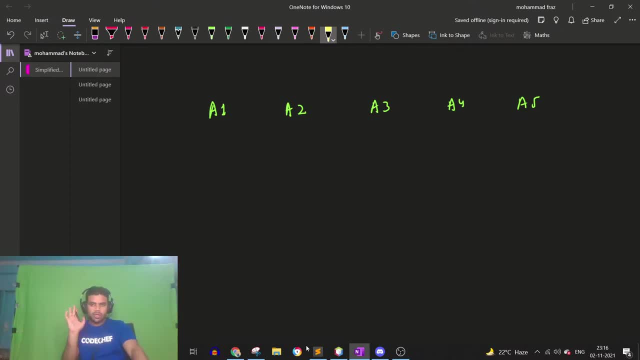 we can select maximum number of activities according to this. we have sorted them, got it. now we have to maximize our profit. we have to maximize the profit. now what we will do, we are going to find the maximum profit that we can make a particular point till a particular activity. 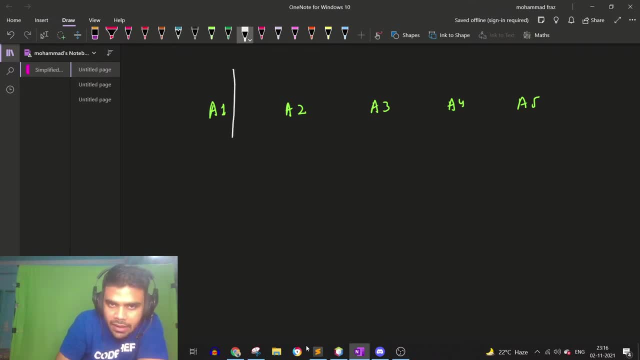 how much profit you can make. activity number 1: till here, how much profit you can make. can you tell me what is the maximum profit that you can make? till activity number 1? forget that other activities exist. till activity number 1: how much profit you can make. 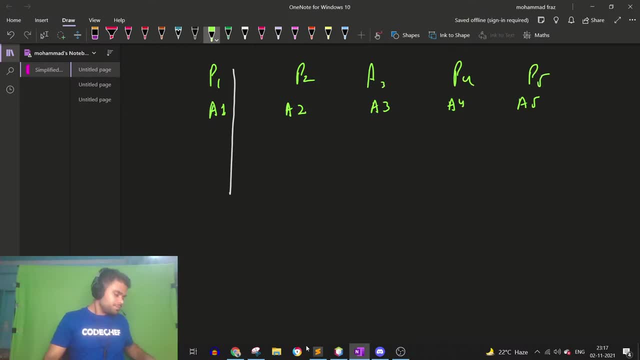 assume their profits are like this: P1, P2, P3, P4, P5. tell me the maximum profit that you can make till the activity number 1. the maximum profit that you can make till the activity number 1, absolutely correct, everyone. 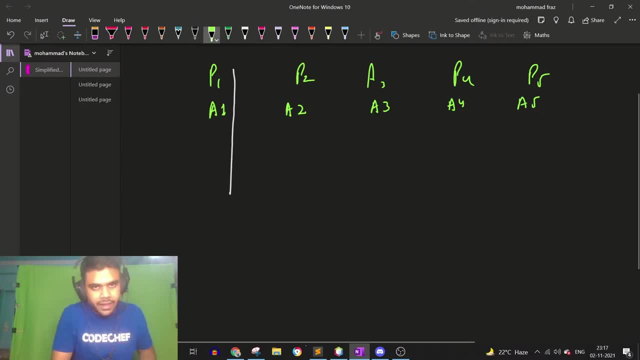 P1 is the profit that you can make. correct, everyone is right, P1 it is. so this is P1 till P2, till P2. how much profit you can make, tell me till here, how much profit you can make. tell me. tell me, we cannot say P1 plus P2. 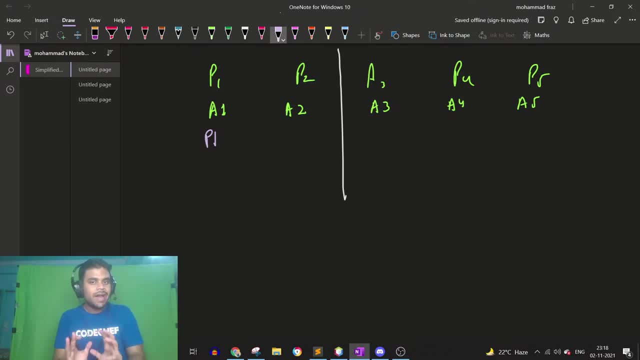 we cannot say that P1 plus P2. why? because it is overlapping, it can be overlapping. P1 and P2 can be overlapping. is there an overall between A1 and A2 overlap? I don't know. that is what I am asking you to do. 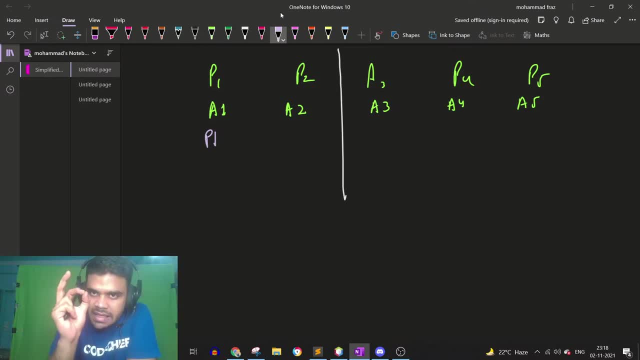 see, I have two options. I have two options. first option is that either I select this activity. second option is that I don't select this. second option is that I don't select this. listen carefully, this concept will be clear to everyone. ok, ok, pay attention, be focused. 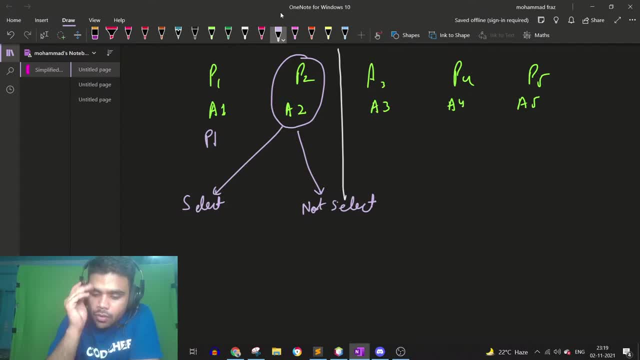 either I select this activity or not. ok, if I don't select this, let's say I am not selecting this particular activity. I don't select this activity. what will be my profit? tell me what will be my profit till A2. till A2: what will be my profit? 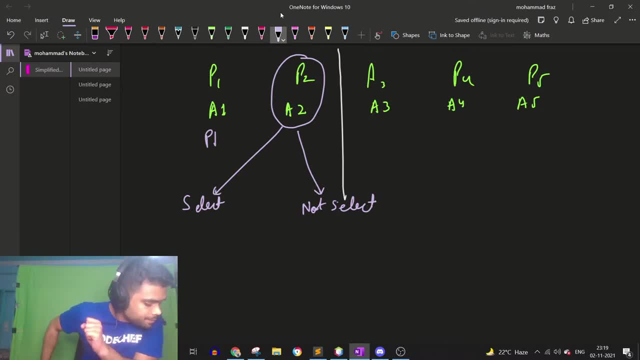 if I do not select the activity A2, tell me some people are thinking in a good direction. let me generalise this idea. ok, let me generalise this idea in front of you. absolutely correct everyone: Chandan Shubham, Akshit Raunak, Yash Shivansh. 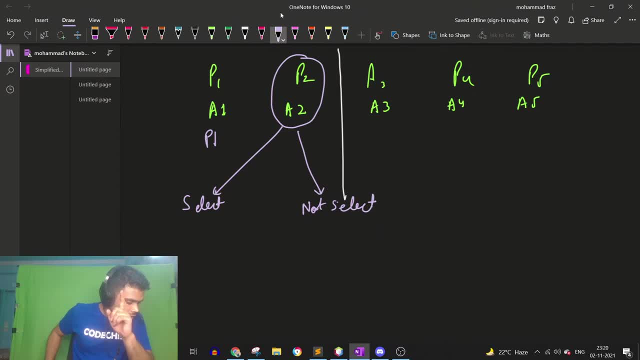 ABC. EFG correct. Saurav Mandal correct. P1 is going to be the profit Means. if I don't select the next activity, then my profit will be same as profit till i-1.. The profit till i-1 will be my profit. 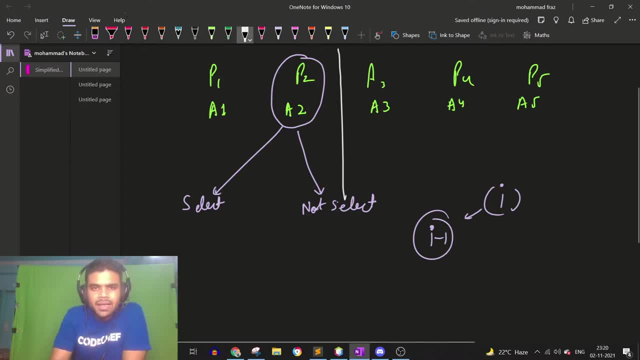 The profit till a particular point is denoted as Pt1.. So what will be the profit till the next point? There are two options: Either I will select the next activity or not. The first option is that I don't select it. 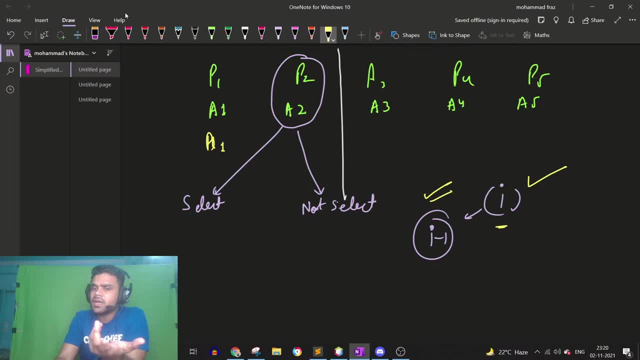 If I don't select it, then the profit till the next point will be same as the profit till the next point. If I don't select it, then the profit till the next point will be same as the profit till the next point. The profit till the next point will be same as the profit till the next point. 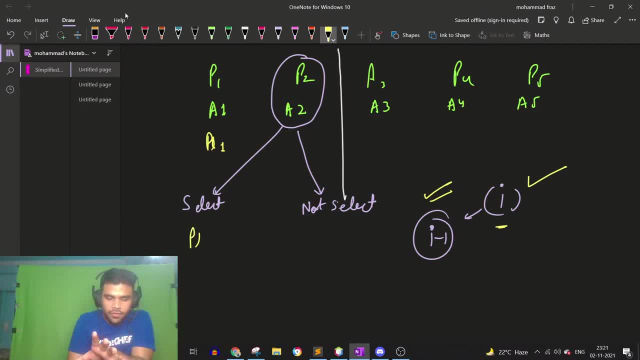 So the first option is that Pt1.. Pt till 1.. Pt till 1.. This is the first option. I don't want to write here. I want to write on not select. Pt till 1.. On not select. 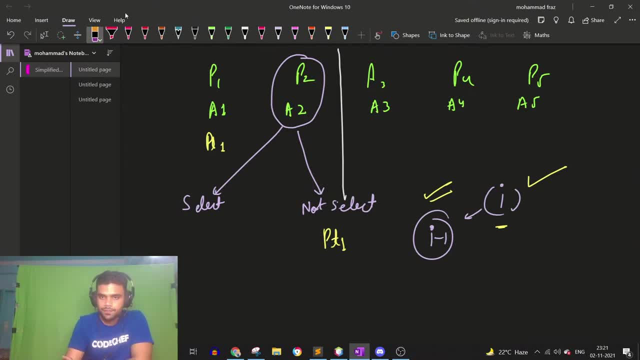 Got it. Did you understand this much? All of you quickly give feedback in the chat. Quickly, Please give feedback. Yes, Yes, Yes, Yes, Akshit, Akshit, you are on the right track. Good, Good, Good. 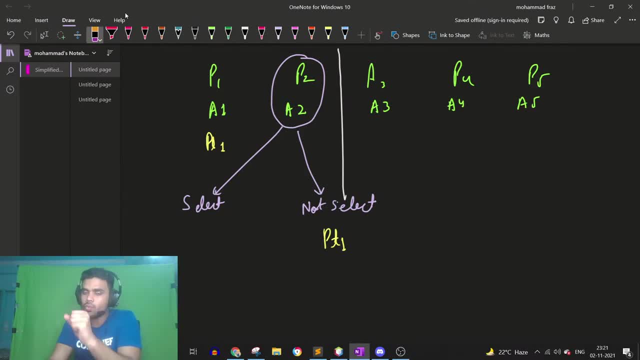 The second option is that I select the activity. Okay, I select the activity. If I select this activity, if I select P2, then it means that the start time of P2, the end time of P2, right, I will have to cover it completely. 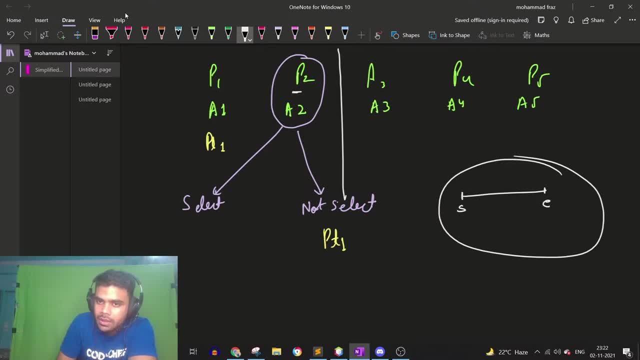 So basically I can say that before P2, listen carefully all of you. Before P2, find such an activity which is ending before the start of P2.. Got it? P2 has been selected. P2 has been already selected. 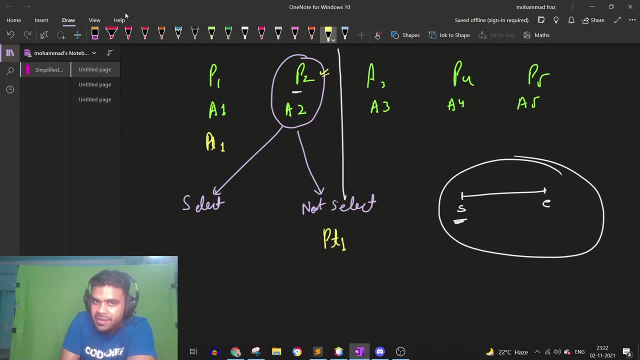 I have selected P2.. So before P2,, go back and forth one by one and see which is such an activity which ends before the start of P2.. You can make a profit up to that activity. You can make a profit up to that activity. 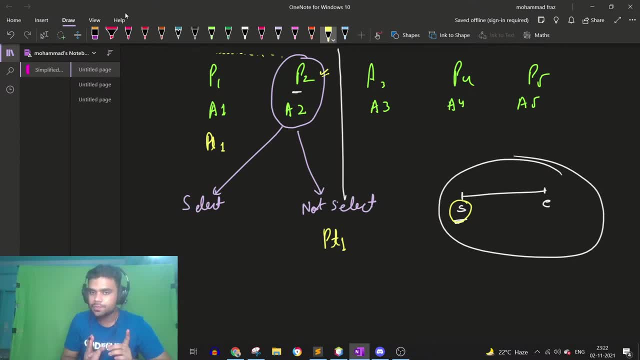 Along with that, you can add the profit of P2 in it. You can add the profit of P2 in it, Got it? So what did I say? I said that if you select P2, okay, Select it, You will get the profit of P2.. 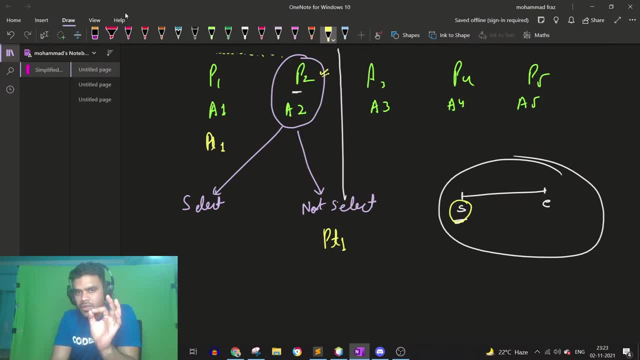 What am I saying about P2? A2. If you can select A2, if you select A2, you will get the profit of P2.. This much profit you will get. Okay, But now you have to go back and check. 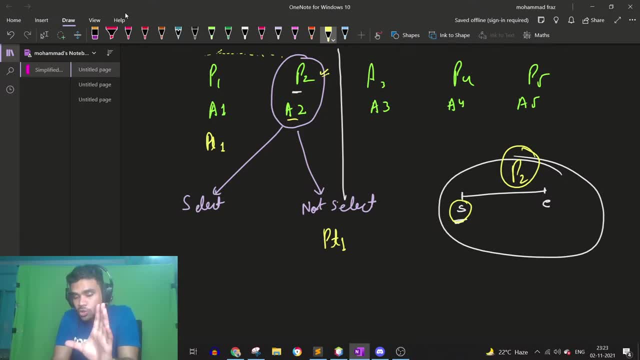 which is such an activity which ends before the start of P2.. So you can make a profit up to that. If it ends before the start of P2, then it will start giving you a profit. You will get the profit after a while. 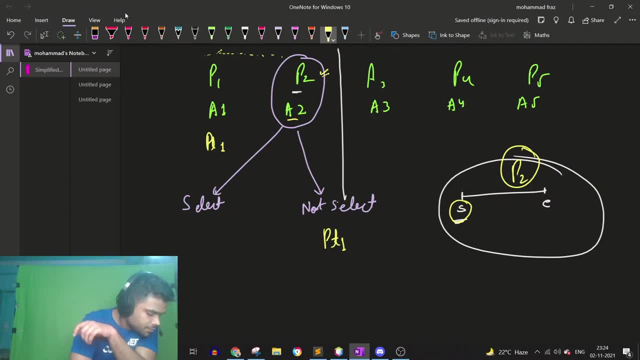 For that you will get a profit. For that you have to. where is backtracking being used? I am telling you, I have to find profit till a particular point, profit till a particular activity. this is it. dp is getting mixed in it, Chandan, did you understand? 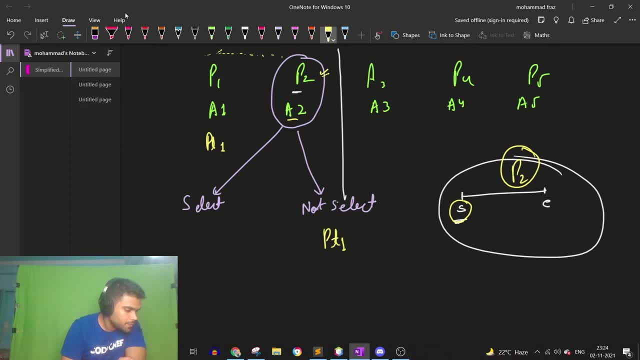 Yash, did you understand? you got into banners. flow breaks with this, not mine. yours breaks to read the flow. you don't understand anything. if you get distracted with such a small distraction, then how will it work? tell me, ok, Chandan nice. 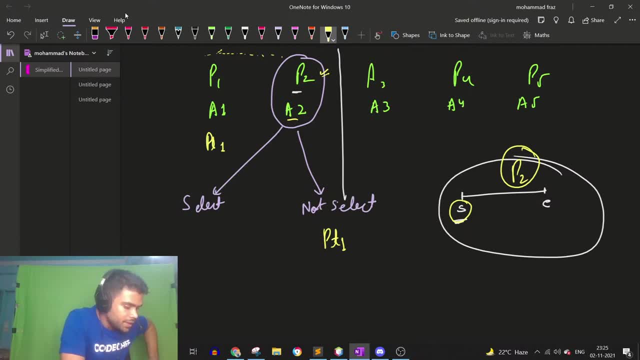 I am repeating it again. we have only 5 minutes left. I am repeating it again. listen carefully. my first option was not to select activity no 2. if I don't select it, then the profit till activity no 1 will be my profit. this was my first option. 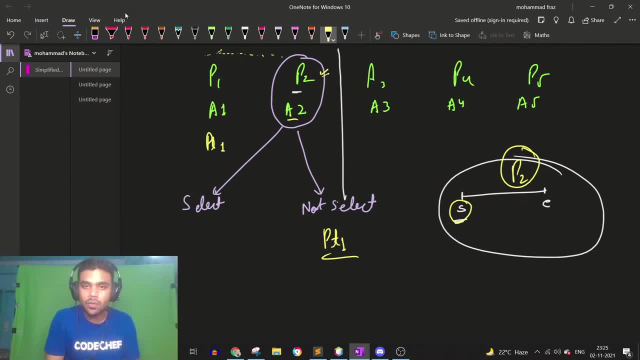 second option: if I select activity no 2, then I will get the profit till activity no 2, but now it is not necessary whether activity no 1 gets selected or not. basically, if I go back and see the time to end of activity no 1, 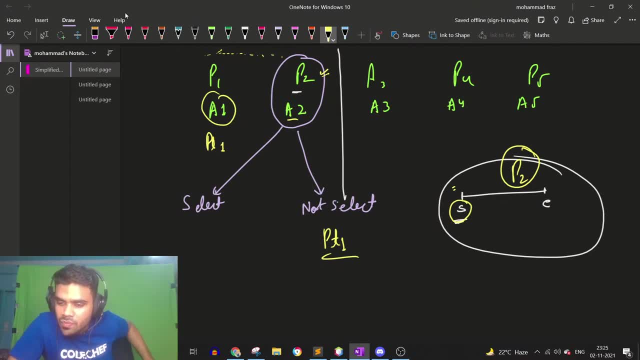 was it smaller than the time to start activity no 2?? was it smaller than the time to start activity no 1?? if it had ended, then the profit till activity no 2 will be added. the profit till the activity no will be added to it. 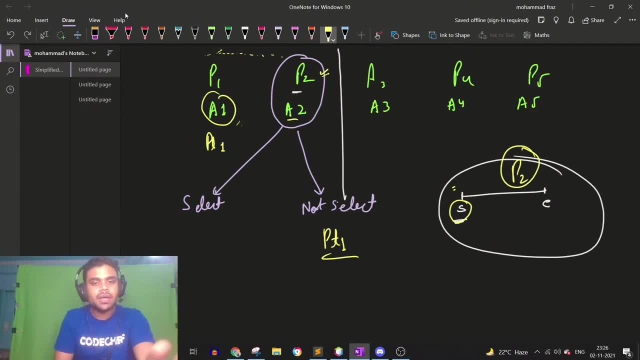 got it nice. so from here the maximum of these two options- suppose this is x and whatever is the maximum of x that I will keep here. so this will be p2. pt2, means maximum profit till the activity. no 2, got it. 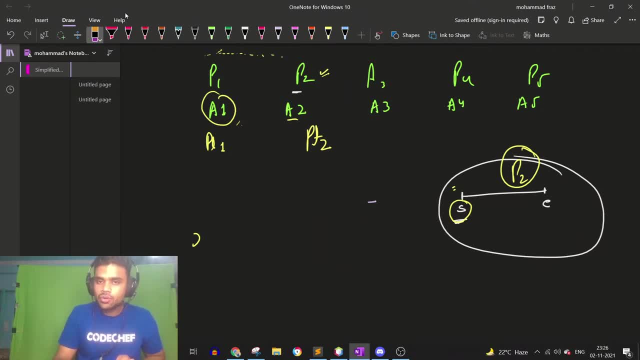 similarly, we will go to activity no 3 and there will be 3 options in activity no 3, sorry, 2 options. there will be 2 options in activity no 3. 1st option will be: either I select activity no 3 or not. 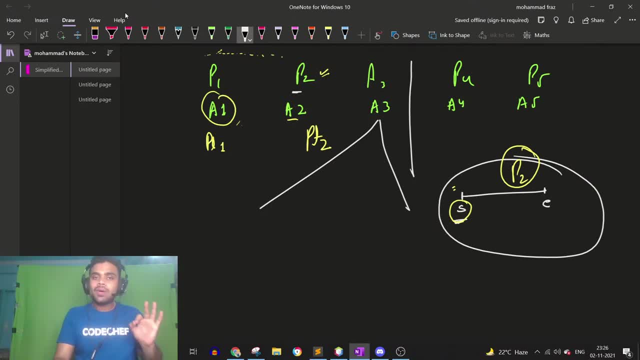 got it. if I don't select, what will be the answer? the answer of activity no 2- that will be the answer- means profit till .2. this will be the answer. this is my 1st option, Profit till 2, and if I select it after selecting, 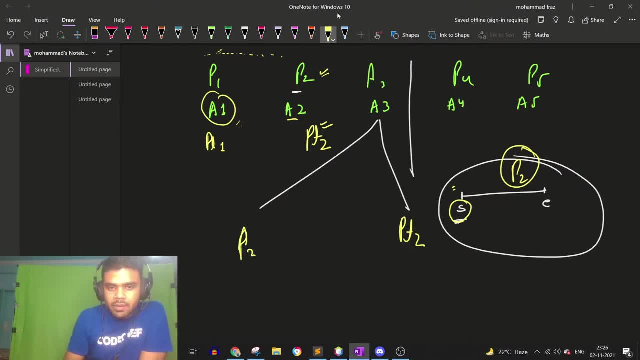 in it the Profit no 3 will be added, that the PROFIT of Activity no 3 will be added. but it is not a necessity that I will Now. I will start going backward and see which is the first activity whose ending time is less than the start time of activity no 3. 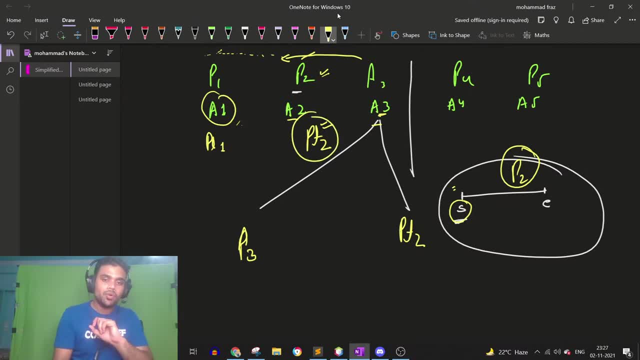 and I will add the profit till that time. profit till a particular j. Got it. So for any index i I have two options. One is the profit till i-1.. The second is profit of i. This is profit till i-1. Got it Profit till i-1.. Second option is: 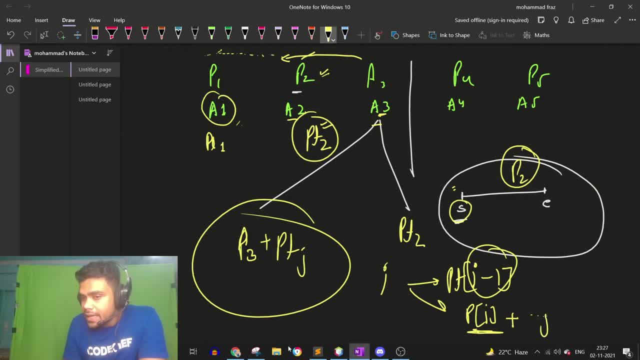 Profit of i plus, we will go backward and we will get a j which is ending before our start time. That activity is ending before i starts. I will take the profit till j. I hope everyone understood. I hope everyone is able to understand. If you didn't understand, then you can repeat the last part. 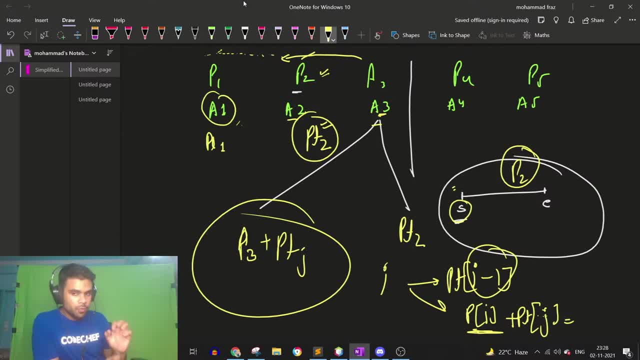 When the video will be recorded, you will get the repeated part. In fact, you can still see. You can rewind the last part, You can rewind it and see. Maximum of these two options is my answer Till a particular point. So my PT5 will be. 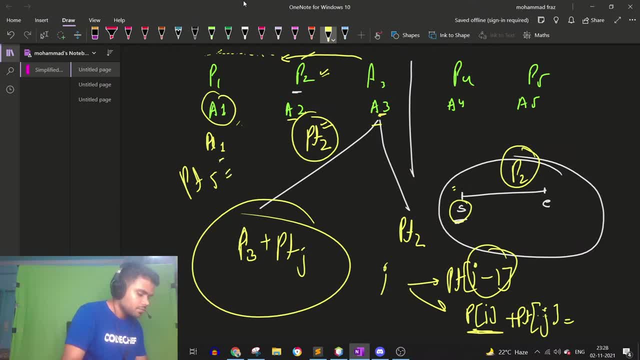 my answer Got it. So you are going backward to find which activity is having the start time smaller than the end time of the current activity. You are looking for such a j, such that the starting time of that jth activity- start of j- is smaller than or equal to end of i. 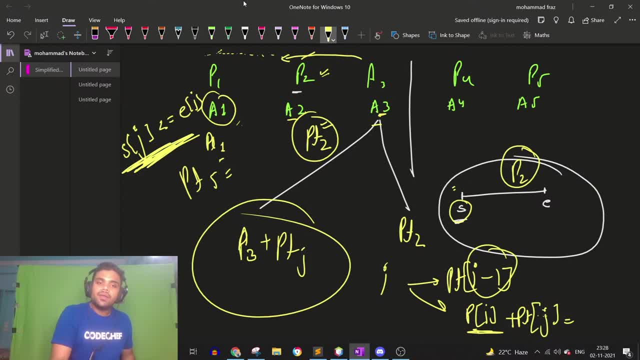 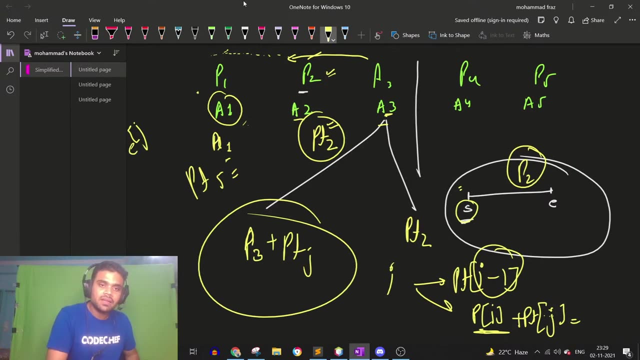 You are looking for such a thing, and you know that I said it wrong. You are searching a j such that ending time of that j is smaller than or equal to the starting time of i. Right, You are searching like this. So here you can apply binary search as well. 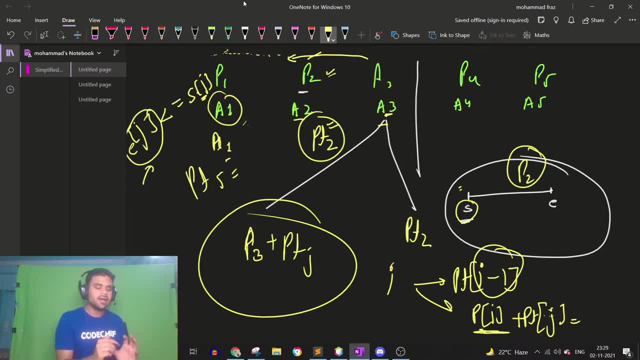 This is sorted according to the ending time. Binary search can also be applied. If you can do it better than linear search, Then you can apply binary search as well. You can search this problem. Name of the problem is Job scheduling with profit. Name of the question is Job scheduling with profit. 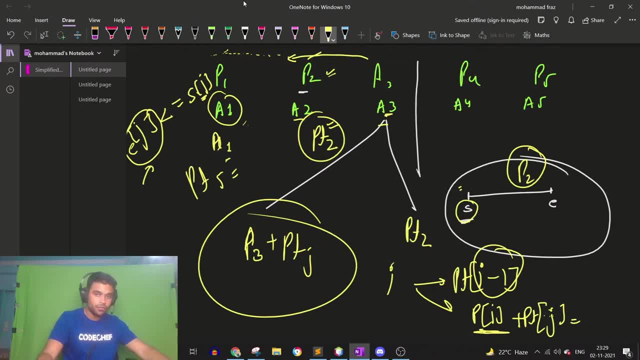 You can search it on google and try solving it. Job scheduling with profit, Let's go. So how was the class? Give some feedback of the class, Like the video. Give feedback of the class, And I hope you are excited to attend the future lectures as well, Which are going to be weekly. 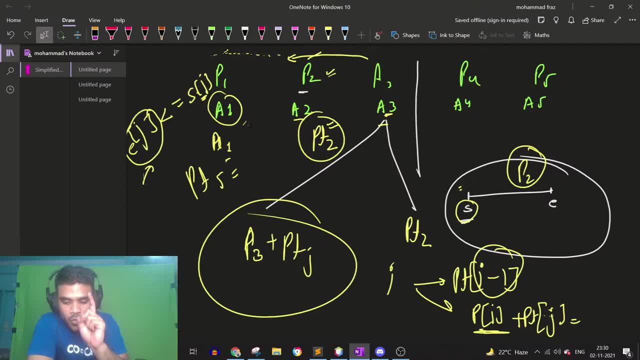 And on Sunday we will have a class of 2 hours In which we will do questions, Most of the questions, Shubham. Thanks, Shubham, Awesome Thanks, Yash And Yash, Don't lose concentration from now. Okay, There is always spamming in the chat. 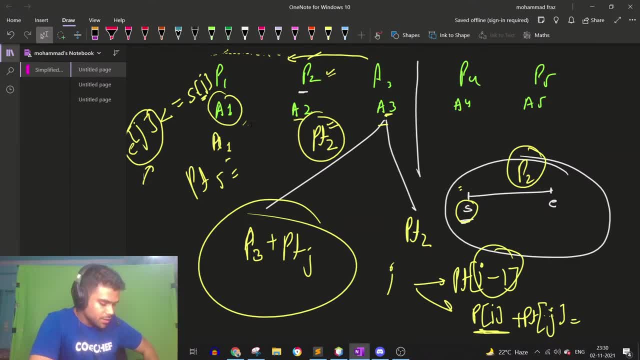 So don't lose your concentration. Very well explained. Thanks a lot, Akshit. This question is not an aggressive one. No, Maybe it is, I don't remember exactly. Thanks a lot everyone. Thank you, A182. Starting and ending same way. Then we should select the activity Which gives more profit. 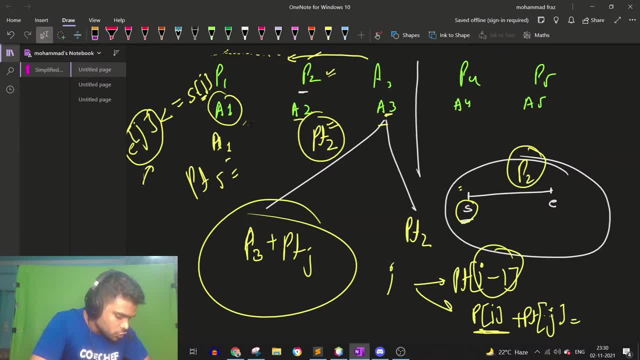 If there is any question, Please answer it in the chat. So the question is: Got better intuition? Yes, developing intuition is the aim of this series. The aim of this series is the same. Okay, Schedule of classes. Classes are going to be held from 9.30 to 11.30. 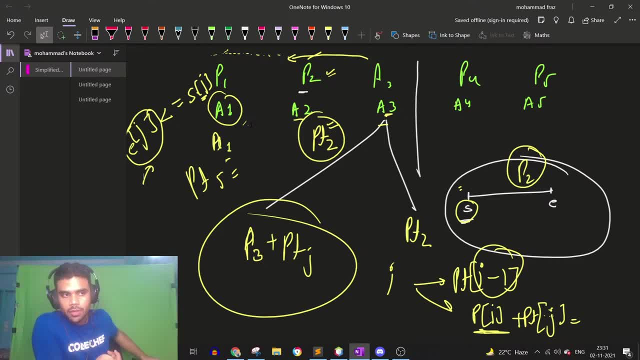 Within the weekdays And on weekend it is going to be held From 2 to 4 PM On Sunday. There is festival on Saturday And on Sunday, 2 to 4 classes. We will keep 2 to 4. Thanks a lot, everyone for your feedback. Thanks a lot everyone for joining. 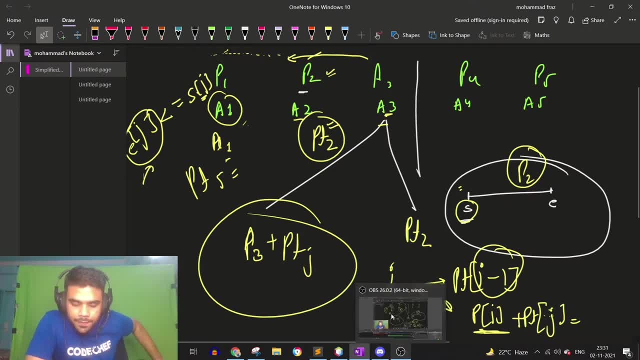 And see you tomorrow. Bye, Bye.